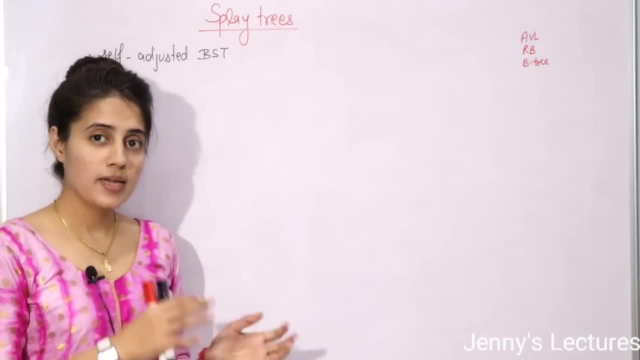 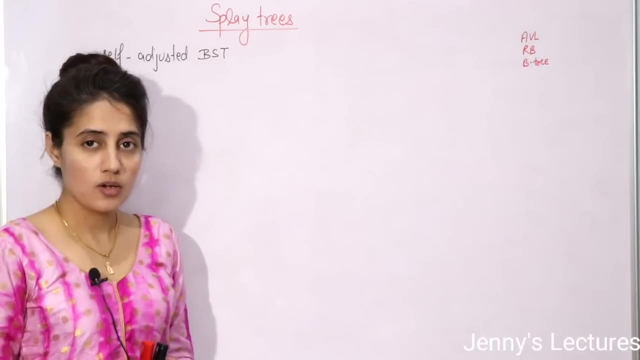 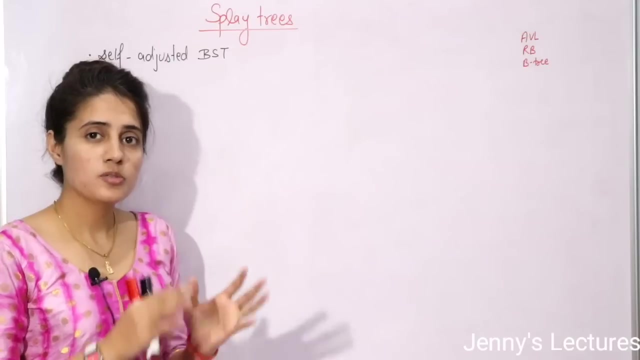 So the topic is splay trees. See, splay trees are basically. these are self-balancing or you can say self-adjusted binary search trees, right, or you can say these are variants of binary search tree. So the prerequisite of this video is: you should know what is binary search tree. 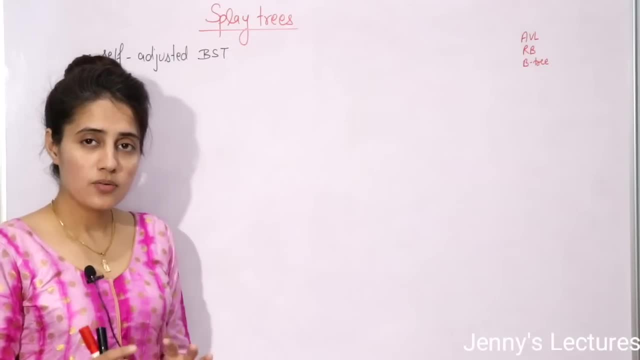 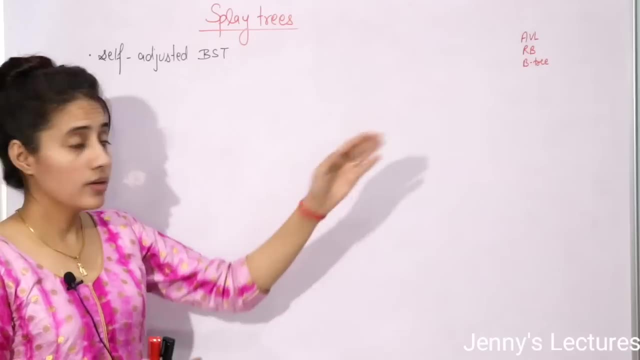 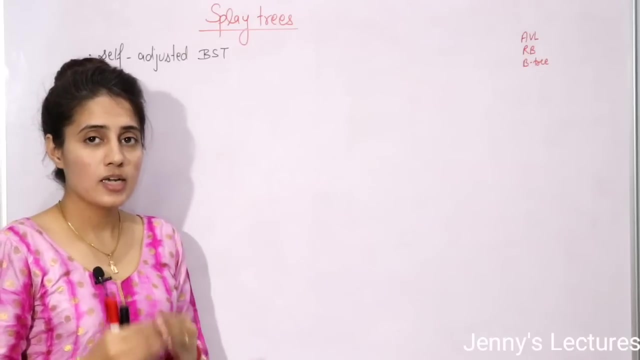 right Now. in this video we will discuss what are splay trees, how splay trees are different from other, balancing binary search trees like avial tree and red block trees, right and as well, as we will see advantages and drawbacks of splay trees and, at last, we will see some applications of 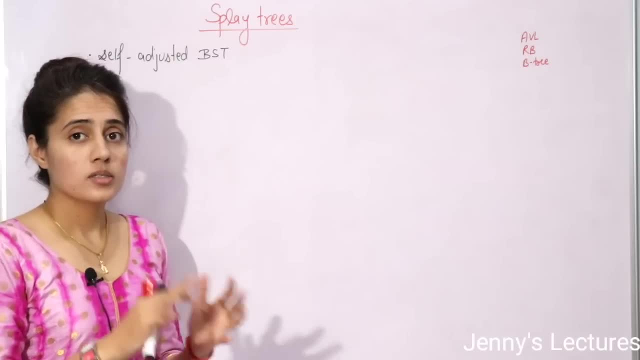 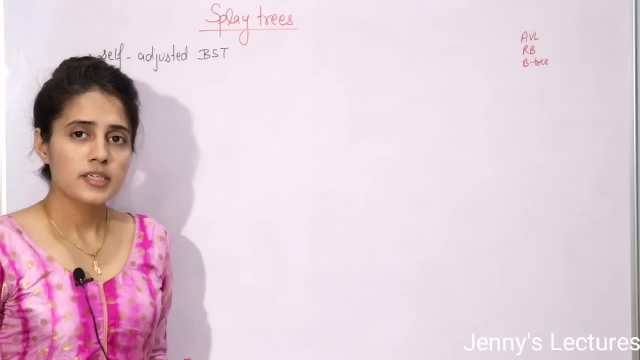 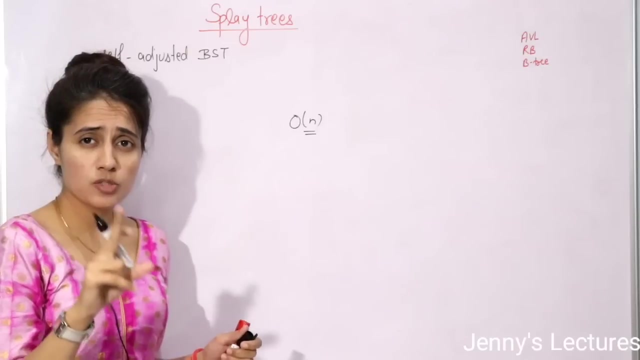 splay trees, right. So now we will discuss what is splay tree. Now see, as we have discussed, in binary search tree the time complexity is what? in worst case, the time complexity is order of n. I hope everybody understood, Everybody know what is binary search tree. In that case, the left subtree of a particular node is: having all the values less than that node and the right subtree of that node is having values greater than that node, right, and in that case the time complexity for all the operations like search, insertion, deletion, is order of log n, But in worst case it can be order of n. Why so? 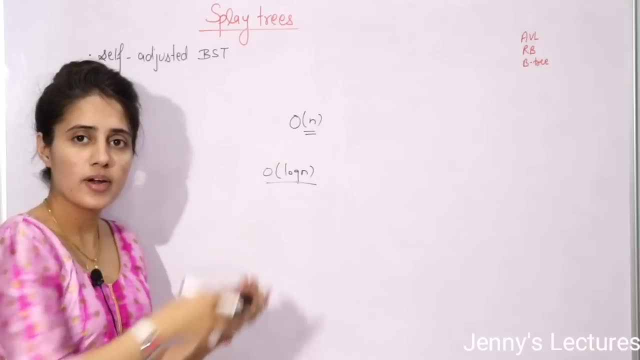 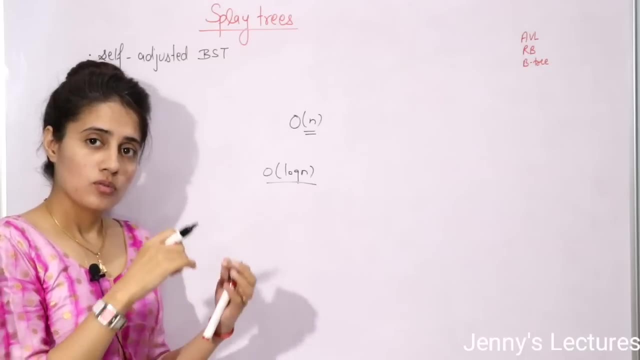 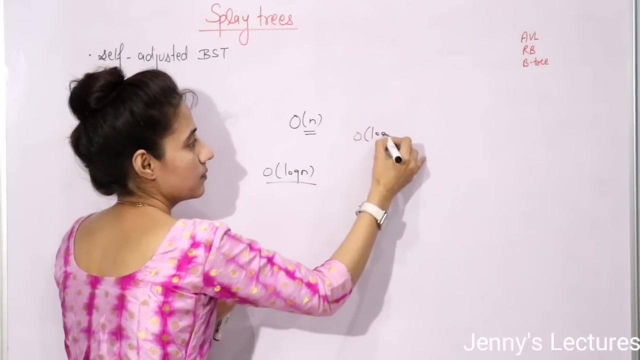 Because if the tree is skewed, either left skewed or right skewed- that thing we have already discussed Right but the time, complexity, in worst case and in average case, at all the cases in avial tree and in red block trees, it is order of log n Means, avial tree and red block tree guarantees that. 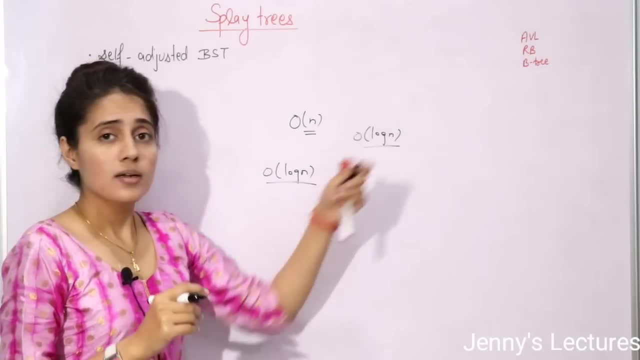 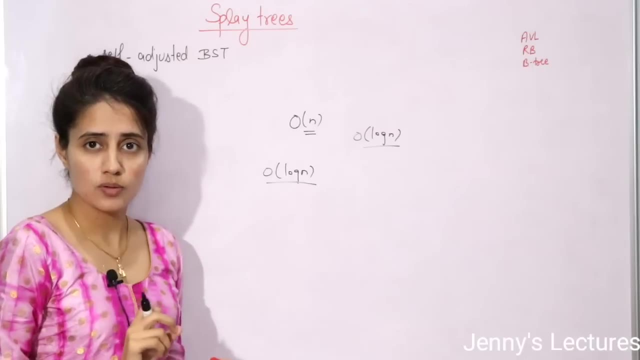 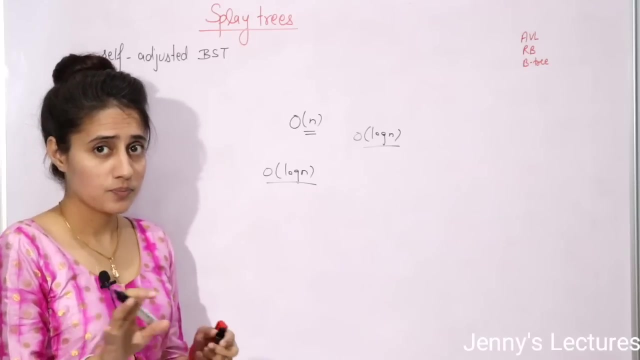 the time. complexity would be order of log n, because these are balanced trees, self-balancing trees. These trees cannot be right skewed or left skewed right. So I hope you have seen my videos on BST, on avial tree and red block trees right. I assume that you know what is BST. 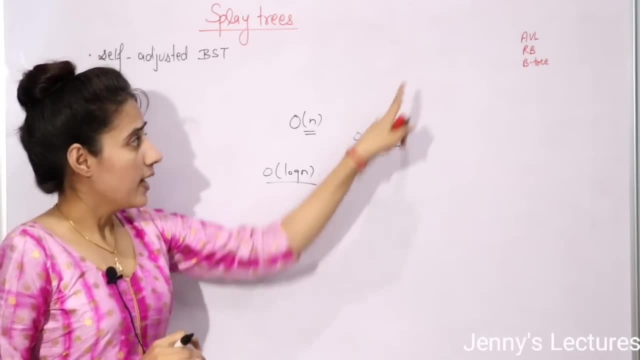 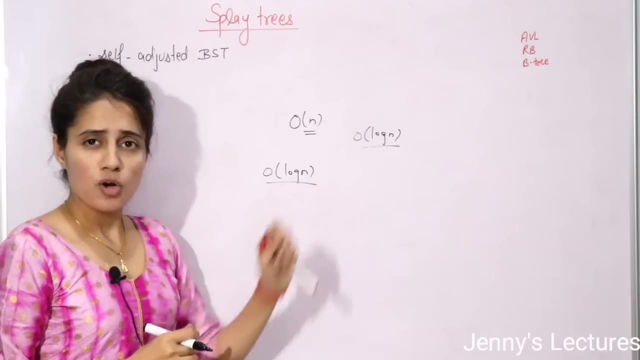 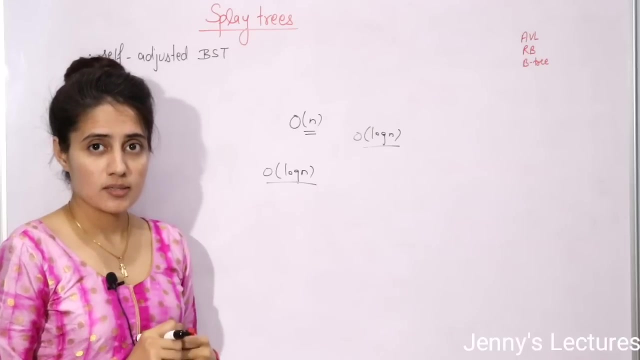 what is avial tree? what is red block tree? right Now, they guarantee that the time complexity would be order of log n for all the operations right Now. can we do better than this time complexity right? In some practical situations the answer is yes, with the help of splay trees. and why the 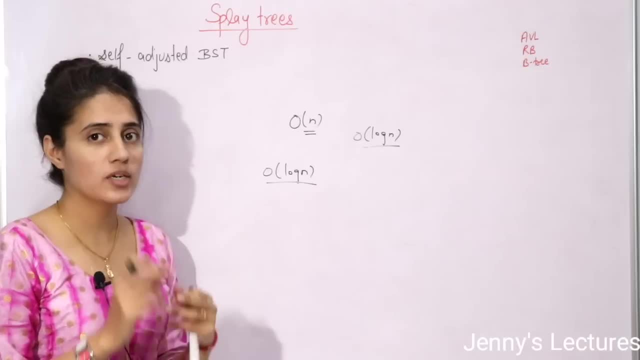 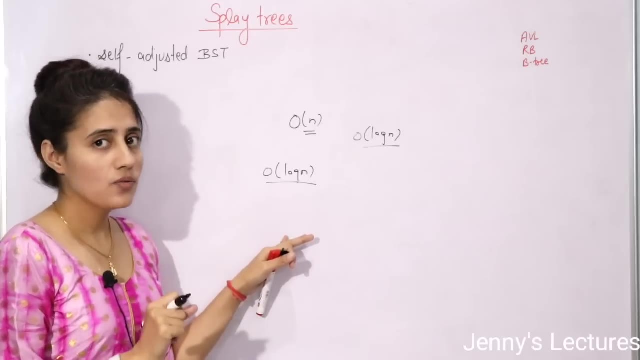 answer is yes, with the help of splay trees. that thing we are going to discuss in the next class, So that thing we will discuss when we will see the advantages of splay trees. First of all, you should know what is splay tree, right? So that thing we will discuss first of all. Now it is, you can say: 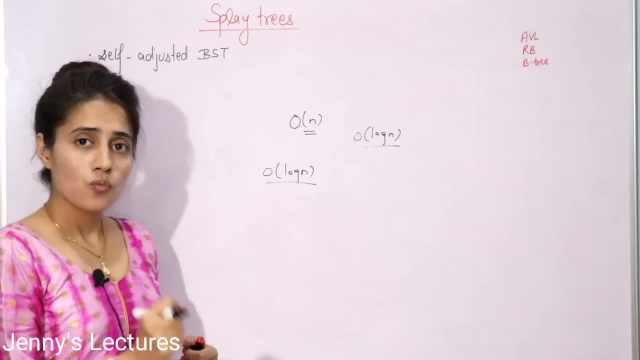 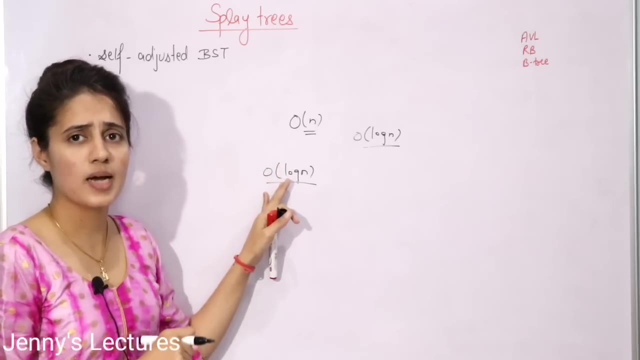 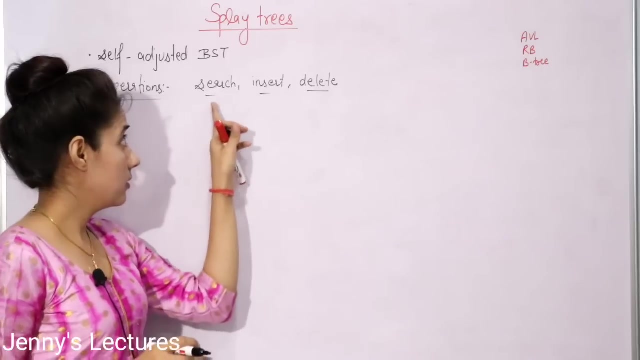 self adjusted or self-balancing binary search tree. plus what extra thing this tree tree have One property is what splaying property? Now, what is that thing? see, see on these trees, splay trees also. the operations would be same as BST tree, like search, insertion and deletion and the process of 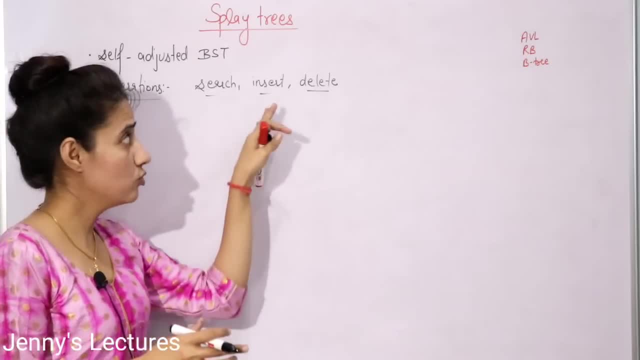 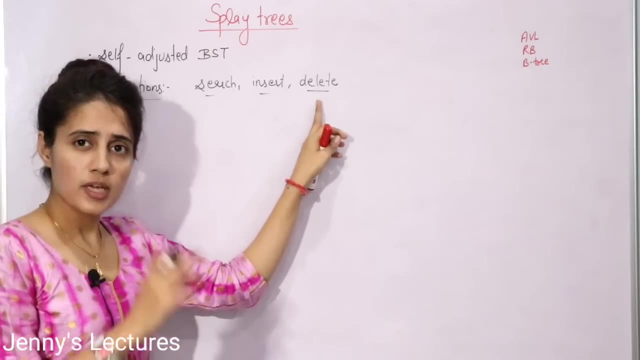 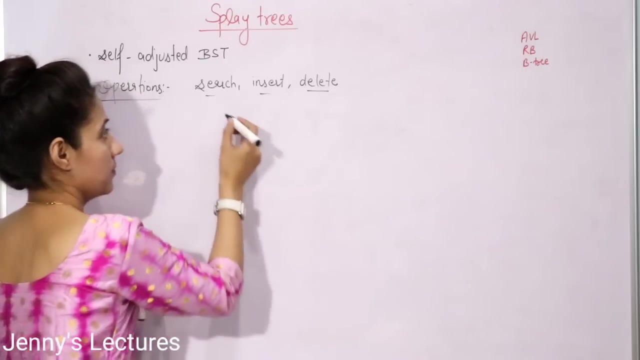 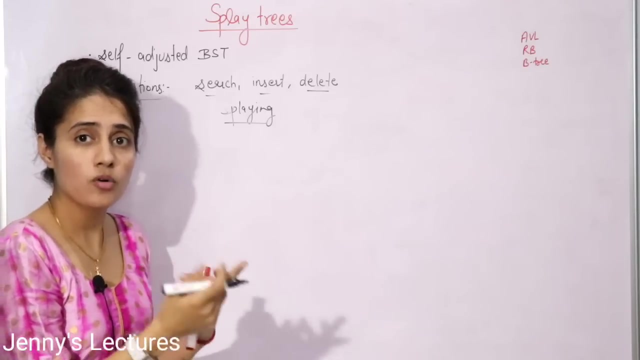 and the procedure would be same as we have conducted these operation in binary search tree, right, plus extra thing is what? here all the basic operations would be same as binary search tree, with some extra operation that is splaying these. all the operations are followed by one operation that is splaying right, this is the extra thing in splay tree. now what? 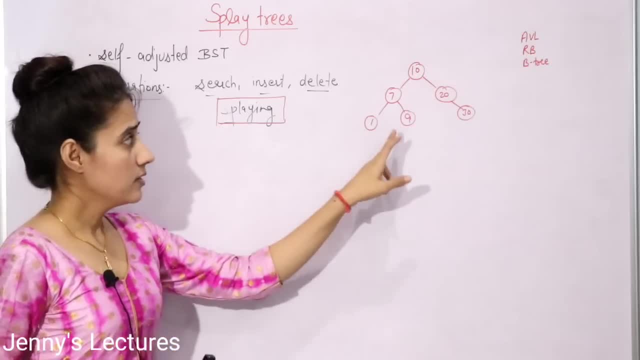 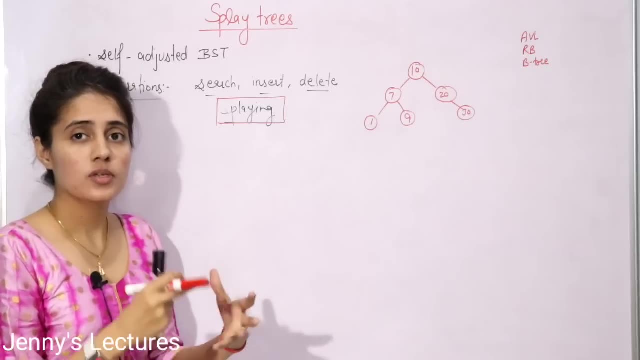 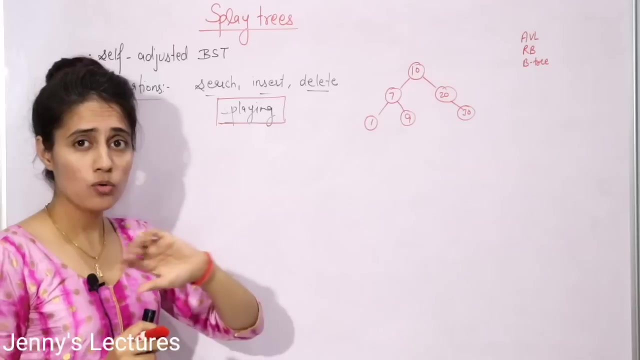 does this splaying means? see, this is a binary search tree. splay tree is also a binary search tree. see, the splay trees are not strictly balanced. these are roughly balanced. avial trees are strictly balanced binary search tree. red black trees are also roughly balanced and these are also roughly balanced tree. fine, now, see, let us take this example. 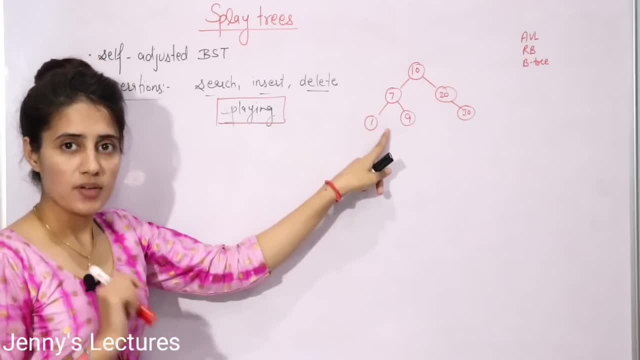 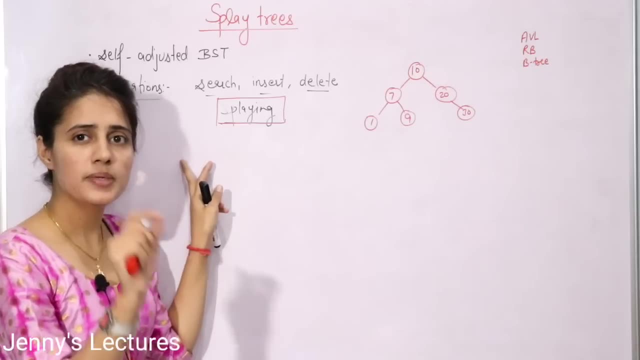 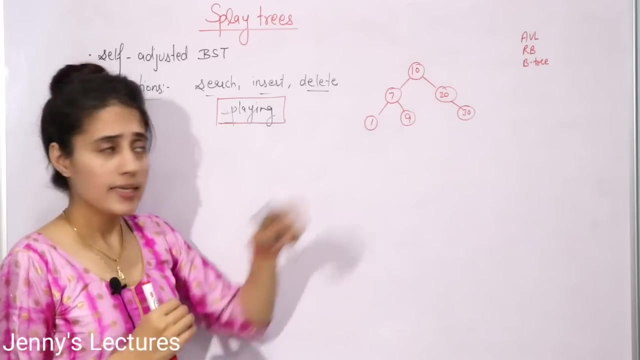 from this tree. i want to search seven, right? so what is the algorithm for search operation in splay tree? just perform standard bst searching. we are going to start from the root because we are having the address of the root node. now seven is less than ten, so we are going. 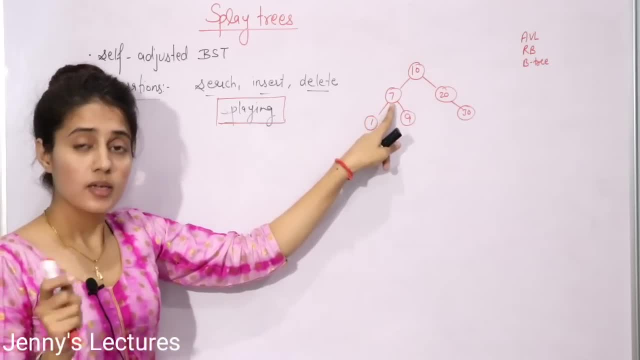 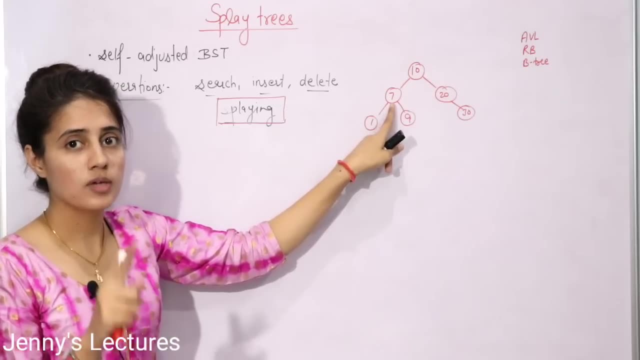 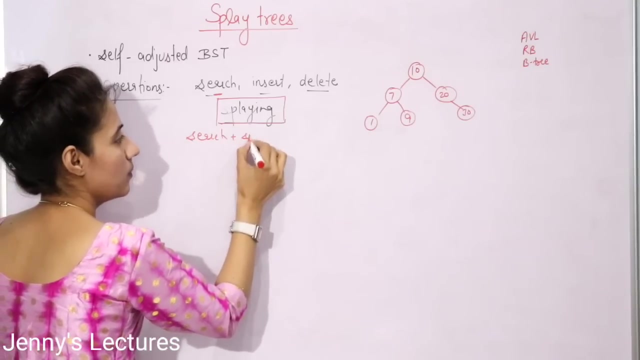 to the left of this ten. here we got seven right. this is what bst searching. now that is done in bst, but here this is not done. the searching operation is not done because here the searching would be followed by splaying. it means search plus splaying, right same insertion. 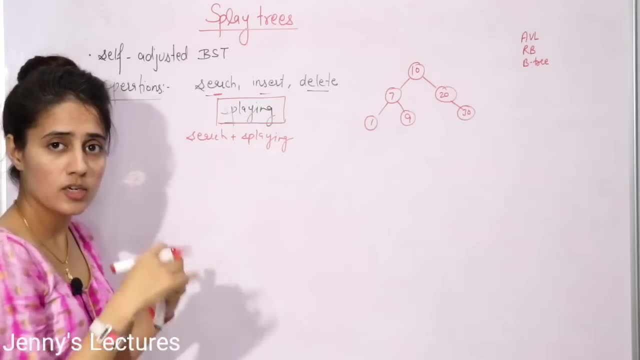 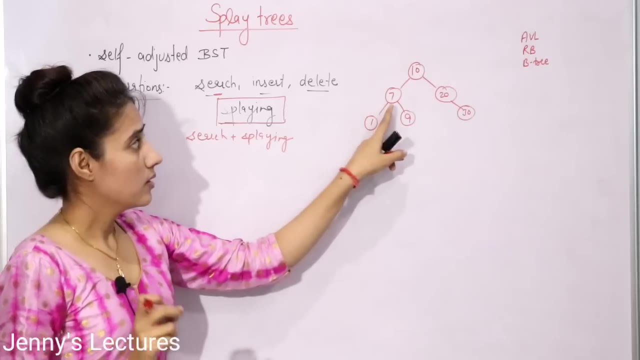 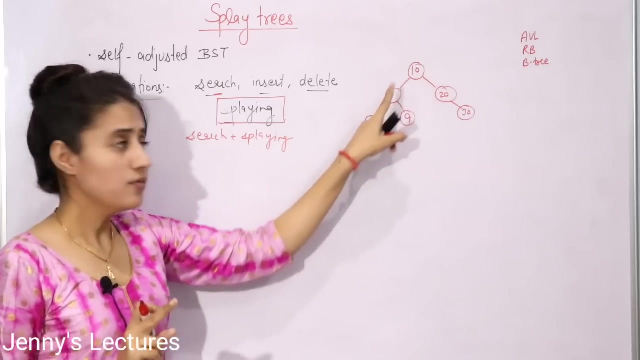 plus splaying deletion, plus splaying insertion and deletion we will discuss in the next video. now, searching is done. now what is splaying? so in this case, we are going to make this seven root of the tree. now ten is the root. after searching, we have found that we have. 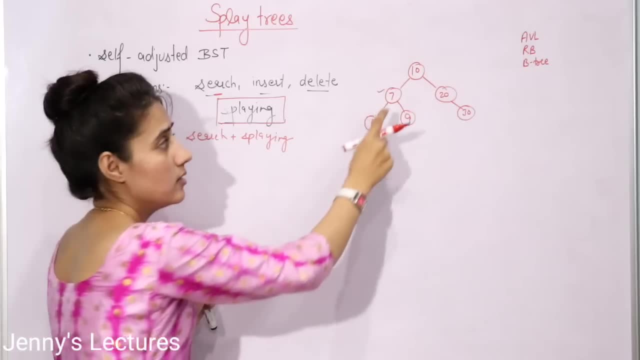 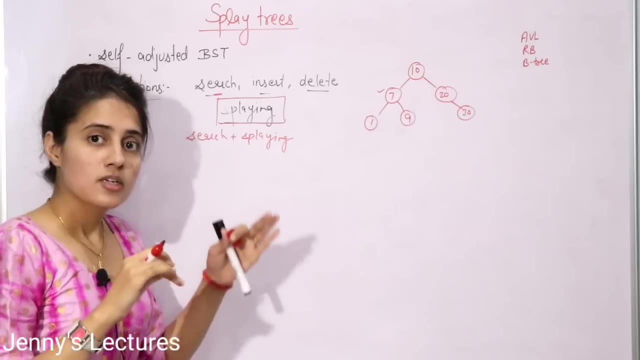 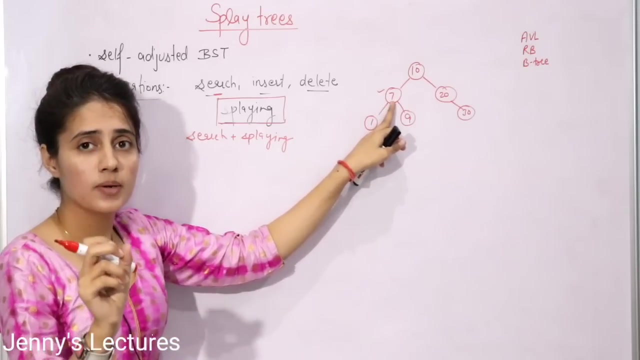 found this seven. now we will do seven. now we will make this seven as the root of this tree. this process is known as splaying means splaying of a tree for this element is what we are going to make: this element or that particular element, as the root of the tree. 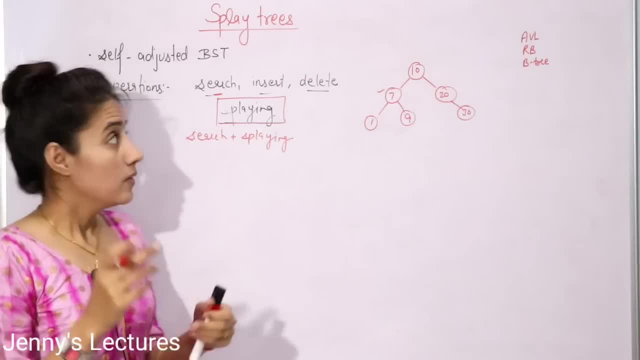 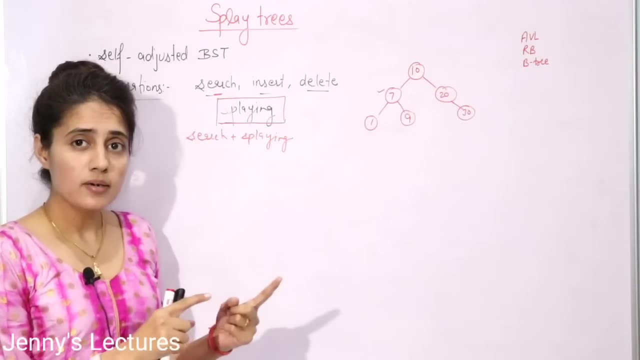 right. so how you can define splay trees. these are self adjusted binary search tree in which each operation of the search tree is a search tree and in this search tree you can find element, rearrange the tree so that that element would be placed at the root of. 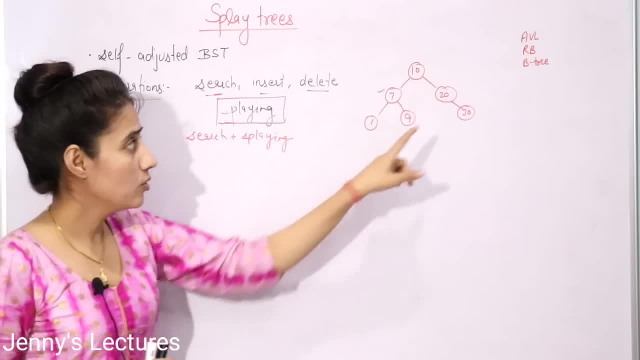 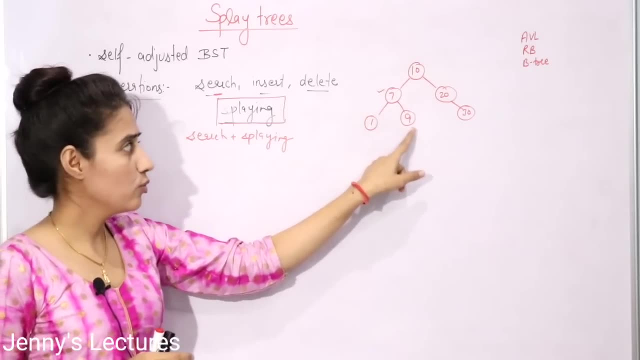 the tree right now. suppose we are going to perform search operation on 9, right. so 9 is less than 10. we are going to the left. 9 is greater than 7. we are going to the right. now. here we go to 9. now we are. we are going to do splang. splang means 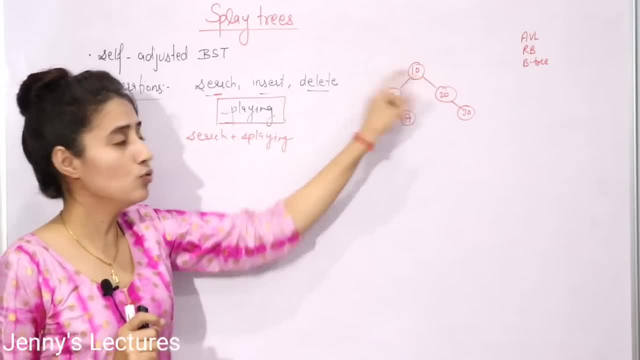 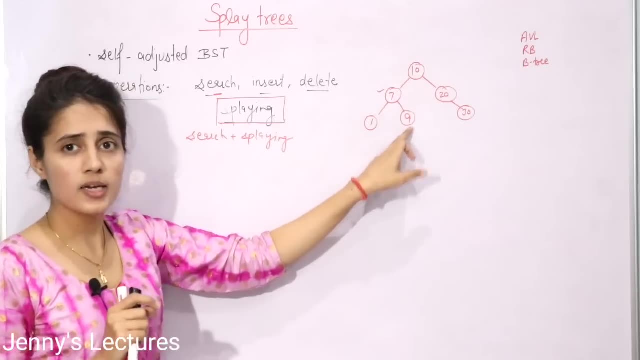 we are going to make this element as the root of the tree. now for making these elements, for suppose I am going to make 9 as the root of the tree. so for making 9 as the root of the tree, you have to rearrange this tree or you have to do. 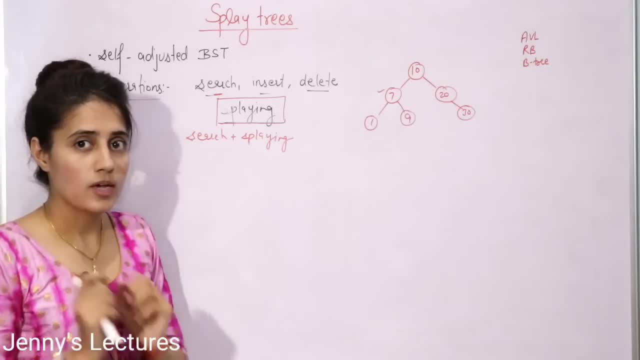 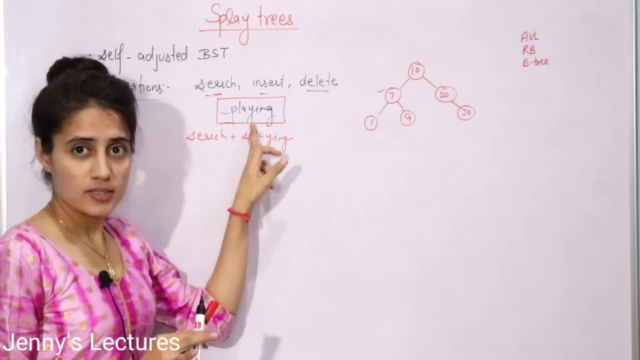 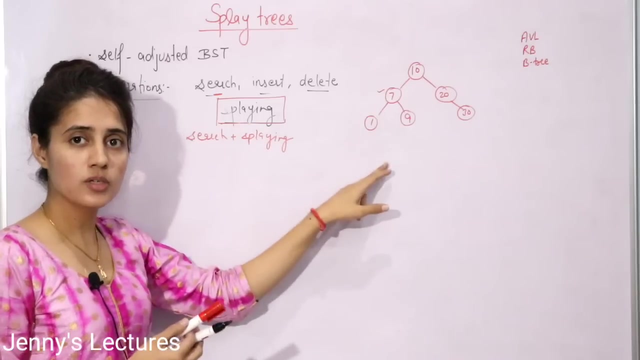 some rotations right now. we will discuss those rotations as well, how you can rearrange this tree to make this as a root of this tree. so I hope you got what is playing in this case. this is the you know, main point in split trees. if you got what is playing- how to do playing of this tree- then it means you are done. 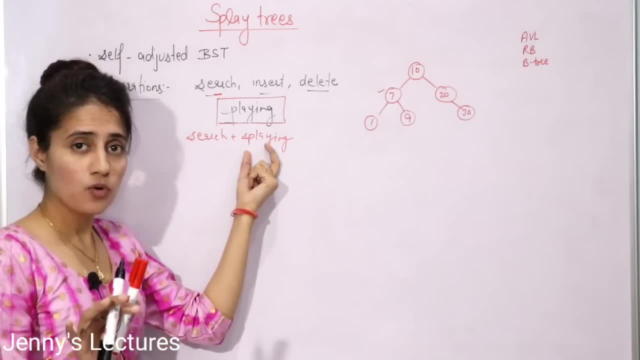 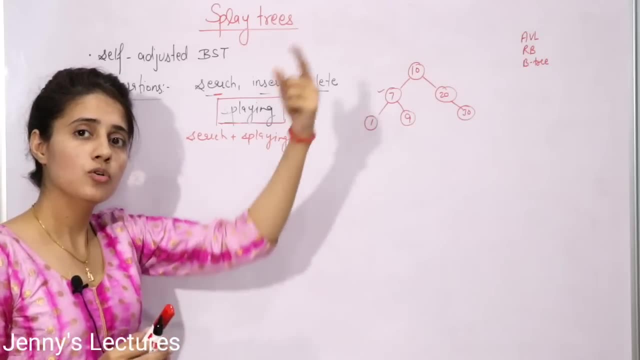 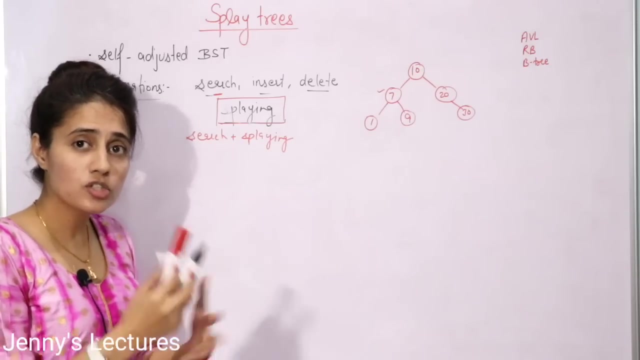 with split trees. you got it right. so splang means basically what? rearranging the tree so that the element on which you are going to perform the operation now become the root of the tree. right, how to do the rearrangement of the tree, that thing. we will discuss the rotations: how many rotations and which type of rotations you 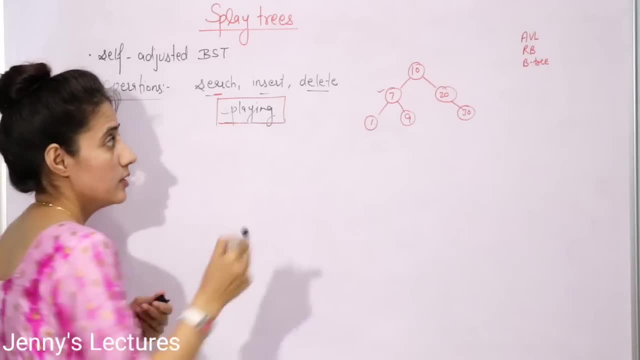 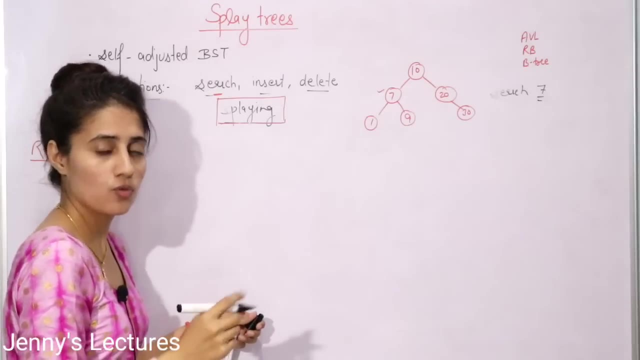 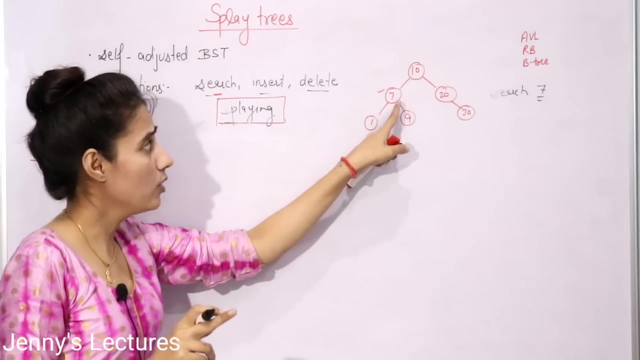 need to perform here right now. suppose we are taking this example and from this tree I want to search 7 right or find 7. you can say 7 is less than 10. so here we got it. now you have to loose playing. now you have. 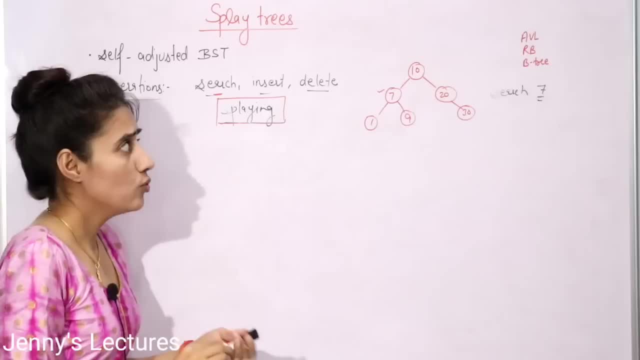 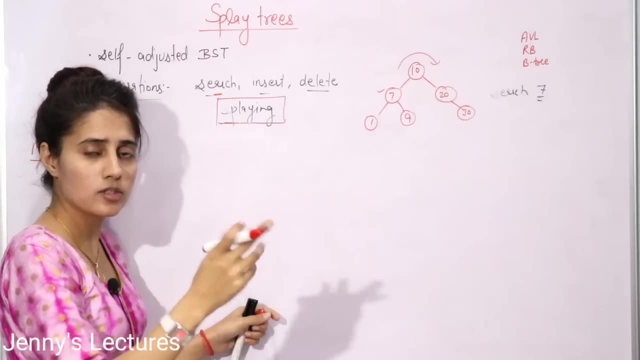 to make the 7 as the root of the tree. so what you can do, we can do right. rotation right, see this. left and right or sheet rotations we have discussed in avial trees. the rotations are same right now. if you do right, rotations means we are. 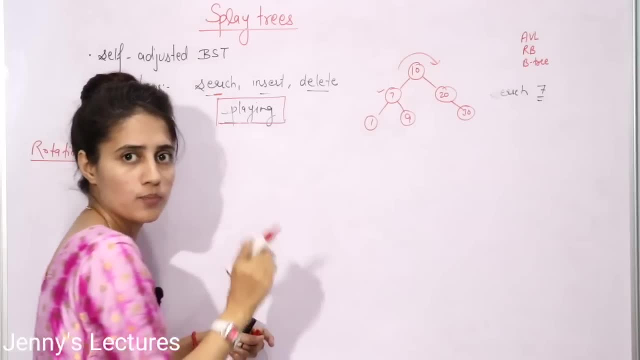 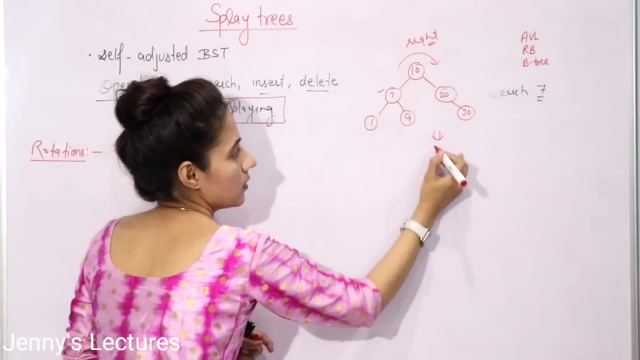 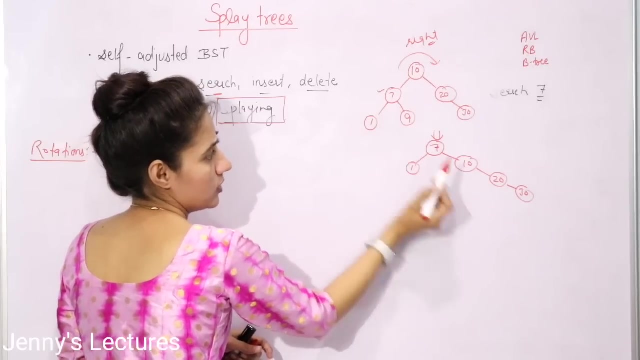 going to push the stand downwards, so seven would go upward right. so now the tree would become something like this in the rotation: now see, the seven is now the root. now the nine is to the right of the seven, to the right of the seven and to the left of this ten, right, so nine is. 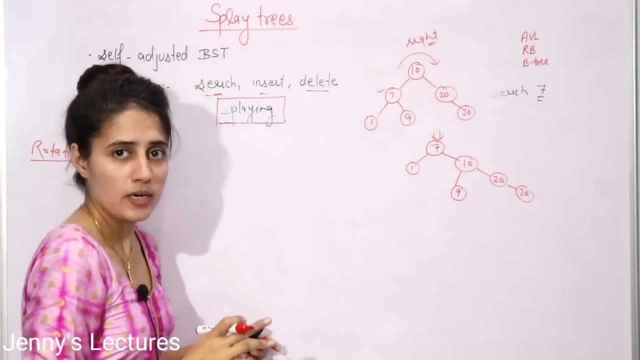 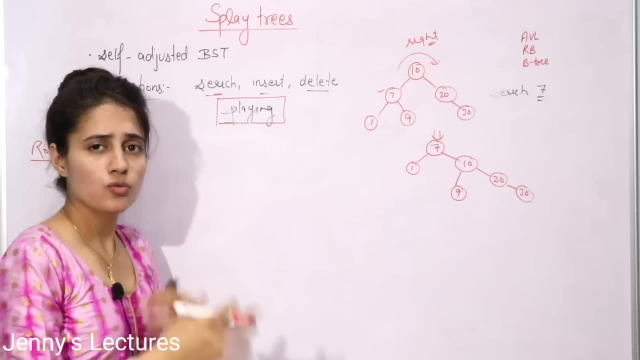 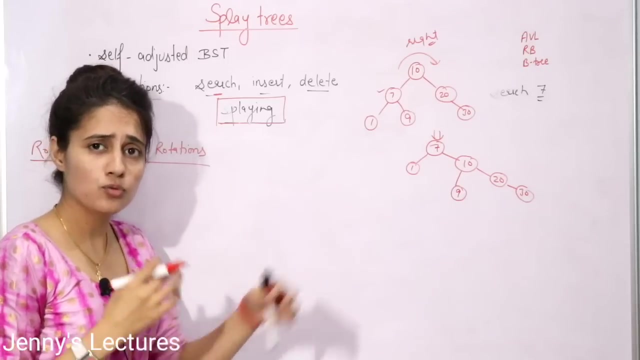 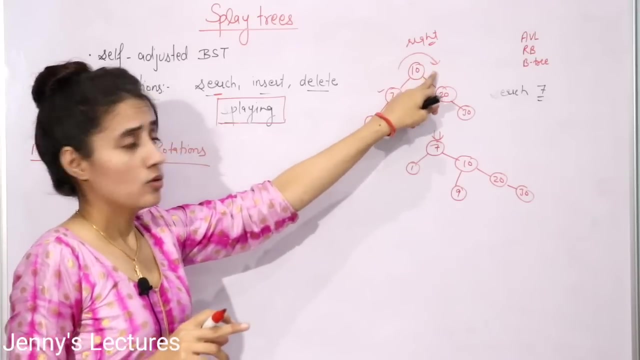 something like this: now, this is the tree split tree after search operation. fine, so now, in this case, this right rotation, or this you can say is known as zig rotation, because for splaying the tree we have to do some steps, or you can say: splay steps, right. so now this, this is what this rotation is, what zig rotations. 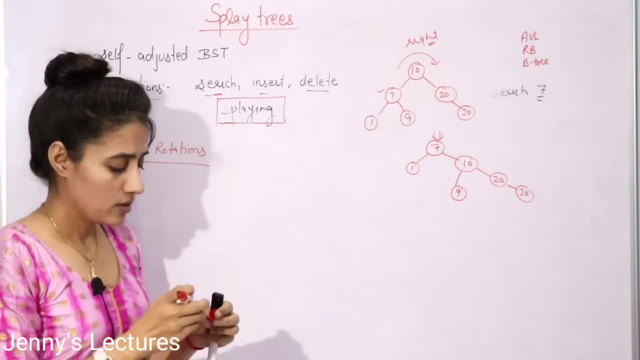 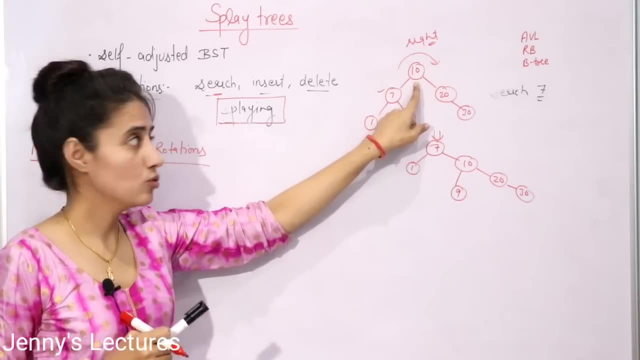 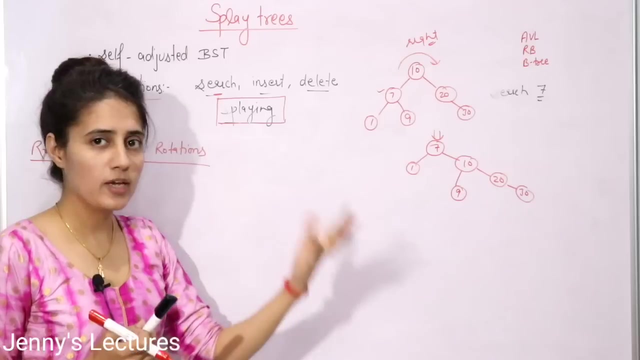 fine, now here the situation may be something like this: see, suppose this situation is: we are going to find ten. now, ten is what the root node, so just, it is already root node. so we are going to return this 10 and we are done. okay, right, no splaying would be done because ten is already root. second scenario is: 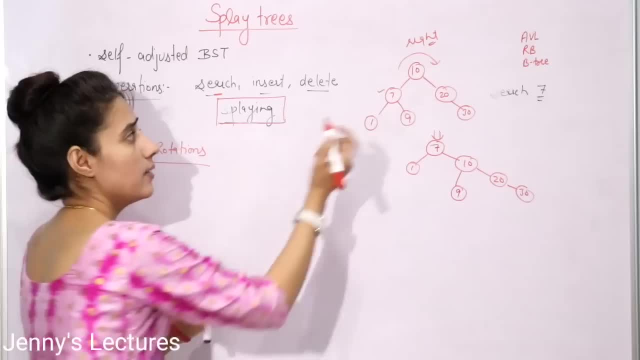 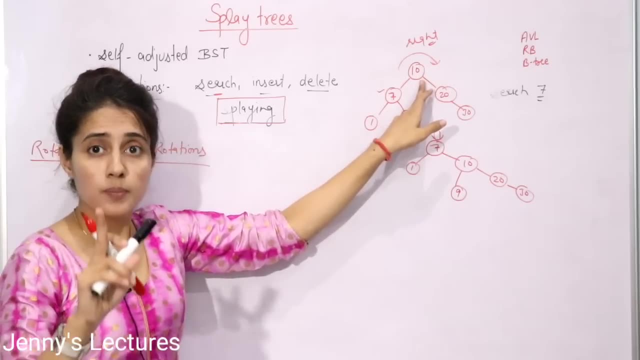 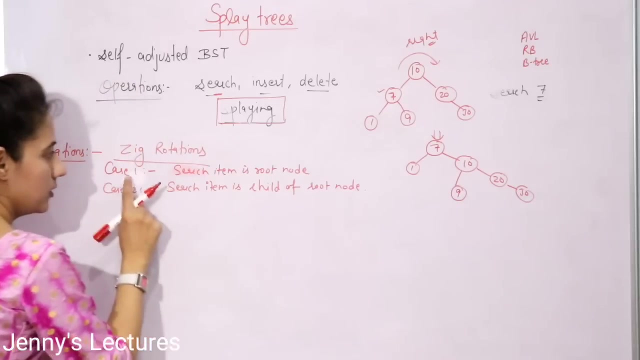 this one. I want to search seven. and this seven, the node you want to search, is child of the root node, means the seven is not having any grand parent. second case: right, see, this is the first case. the search item is root node. just do nothing and return that node now. case second is the search item you want to. 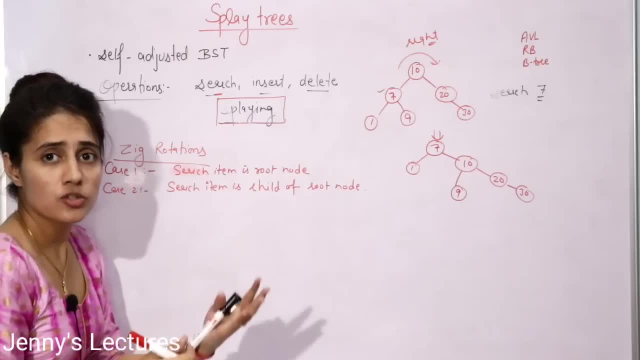 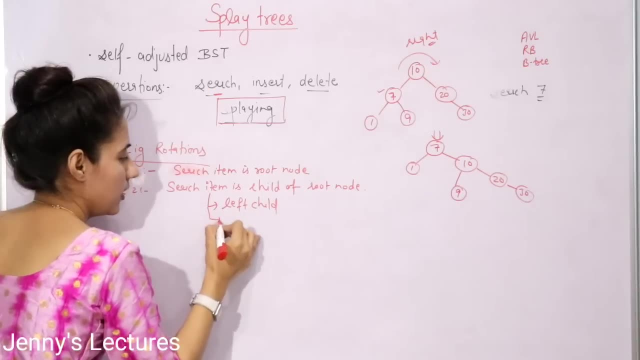 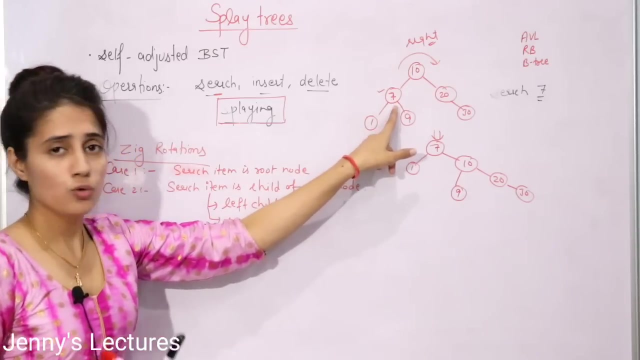 you want to search that element is what child of root node now which child? either left or right. so here also two sub cases can be there. it can be the left child or it can be right child. right now here we have discussed. the item you want to search is the left child of the root. 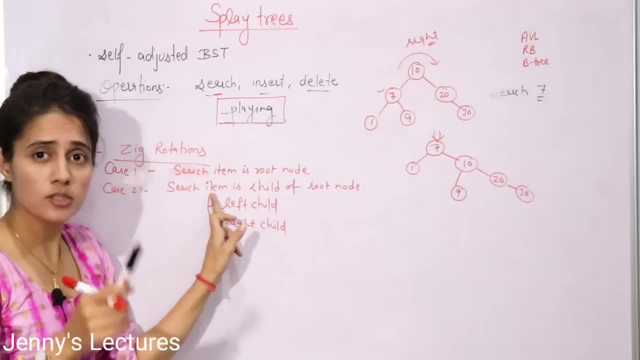 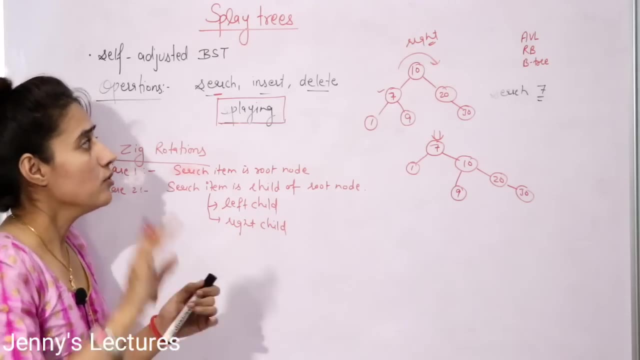 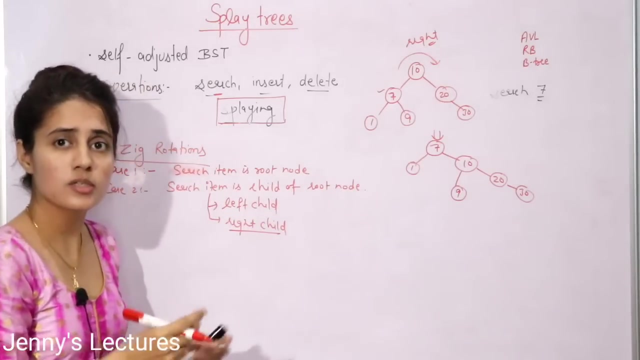 see root node, because the node- it means the node you want to search- is not having any grandparent. this thing you need to take care right now. suppose here i want to search 20 means the 20th item you want to search is right, child of the root node. now what you do. 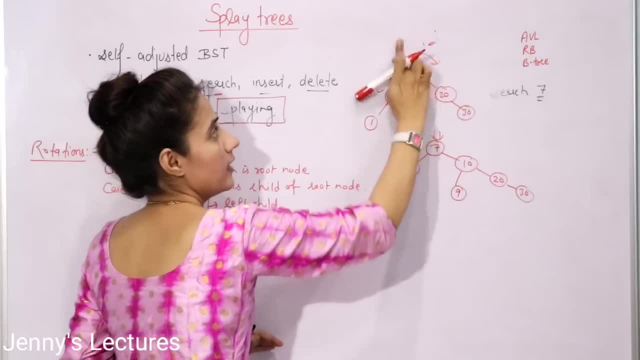 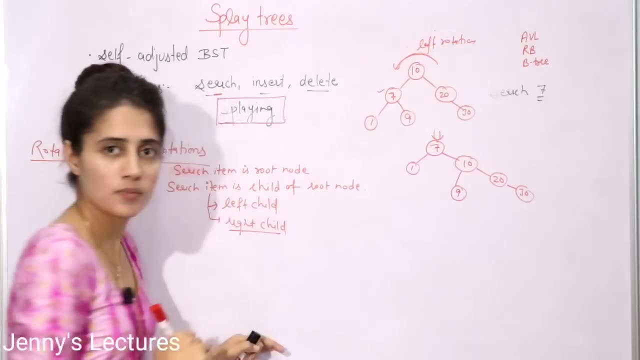 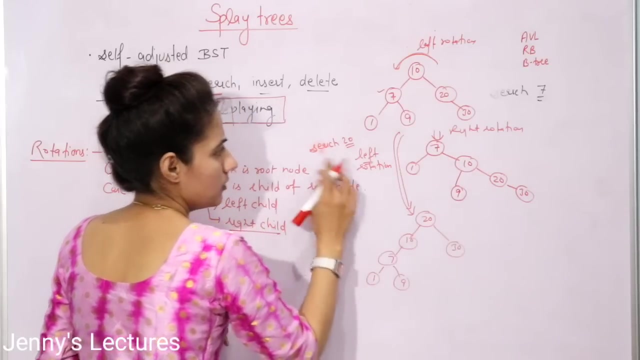 in this case, if you want to search 20, in that case you will do what obviously we will do: left rotation, right and after left rotation. the tree would be something like this: now, this is the tree after the left rotation. see here, in this case we don't have any left child of 20. 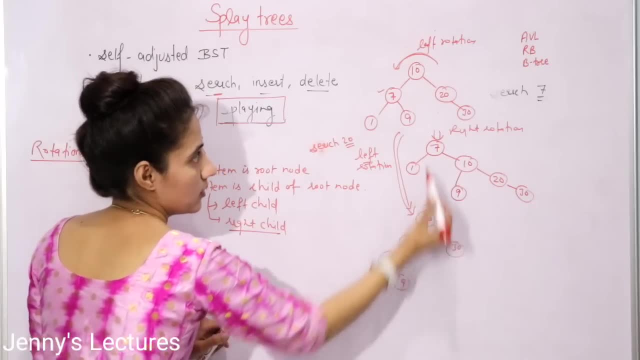 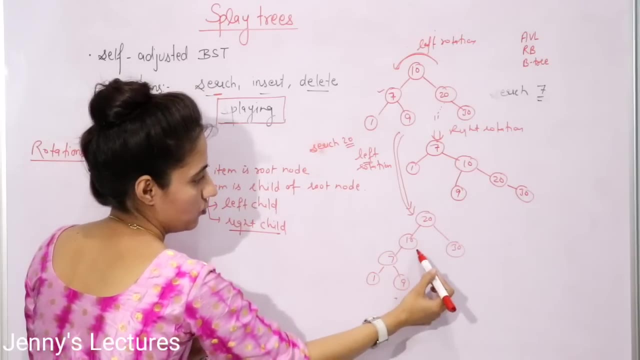 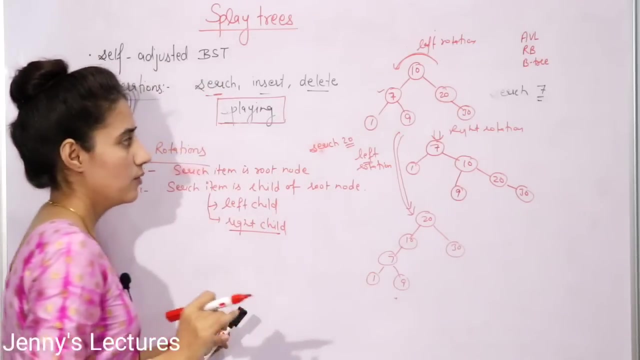 if there would be the left child of 20 means if here we have, suppose, 11, in that case, after this, after this, that 11 would come here. i hope you know how to do these rotations, but we don't have any left child of 20 here. fine, now this. this is known as zeg rotation. 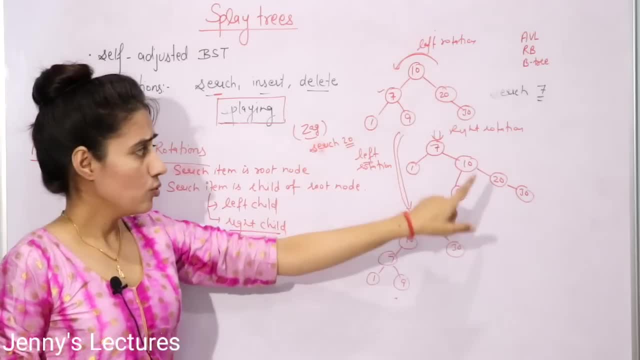 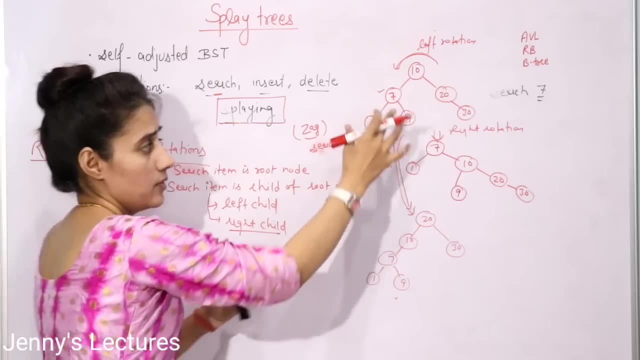 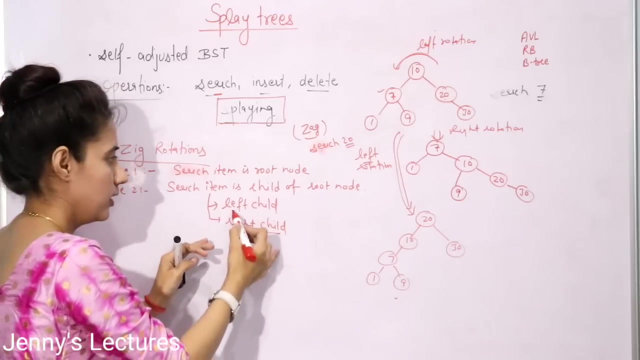 somewhere it is written that this right rotation is known as zeg rotation and the left is known as zeg rotation. fine, but somewhere it is written that this case, if the child, if the node you want to search, is child of the root node, it can be left, it can be right. in both cases it is worth zeg rotation. 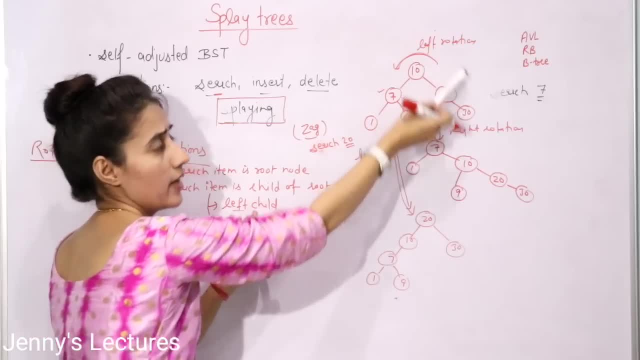 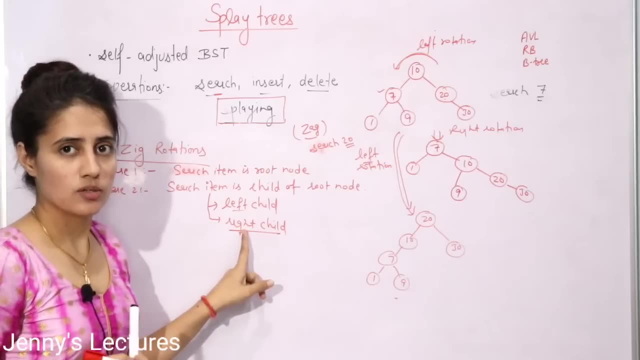 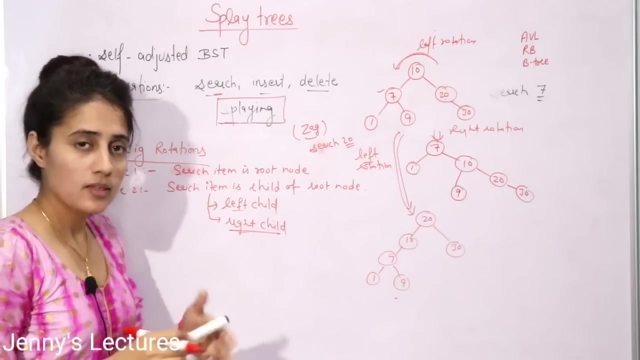 in this case. in this case, if it is the left child, then zeg right rotation. if it is the right child, it is 21, 20 you want to search. in this case it is what zig left rotation? fine, so both the rotations are within the same step. that is a zig rotation, but here in this case, in some cases it is also written. 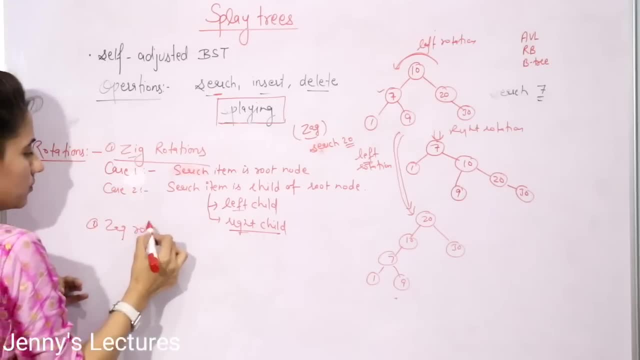 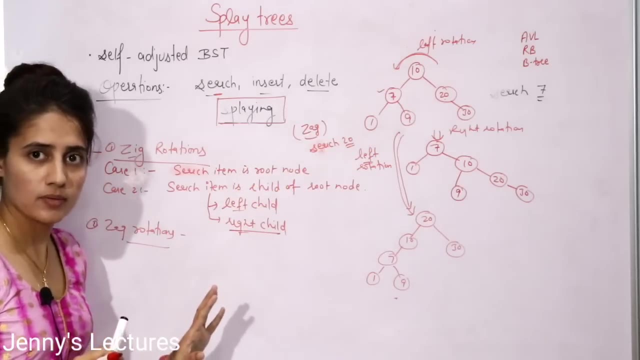 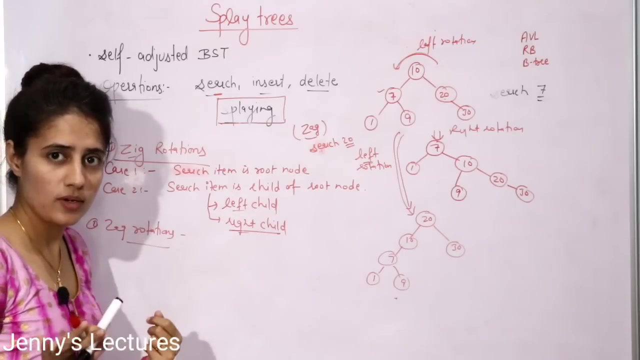 that one is a zig rotation. second is zig rotation. both the cases are right. in zig rotation you can take the right rotation example. in zig rotation you can take the left rotation example right. or you can say: this is zig right rotation or in this case it is zig left rotation. fine, but the 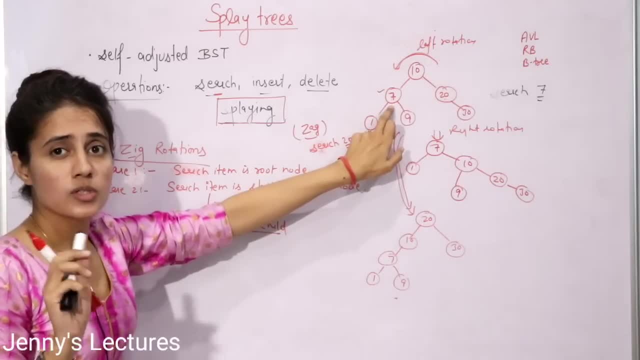 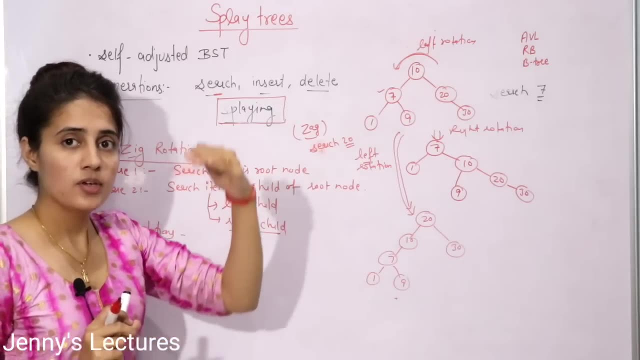 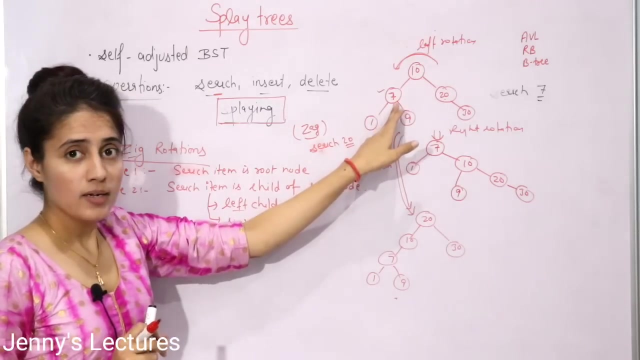 case is this one that. so the node you want to search is child of the root node. now the situation is: if the node you want to search is having parent as well as grandparent- suppose i'm going to search one one- is having parent as well as grandparent. now, in that case we have four cases. 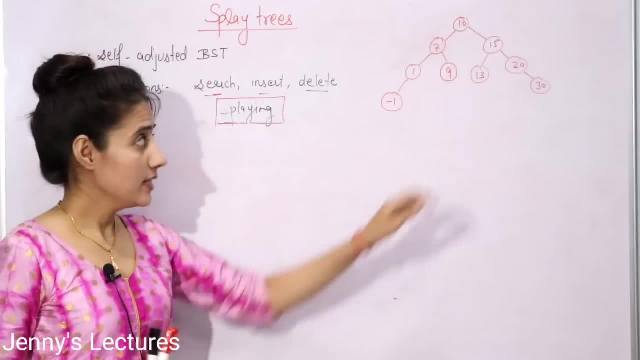 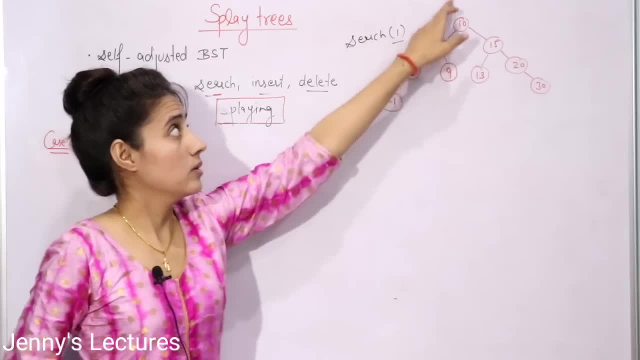 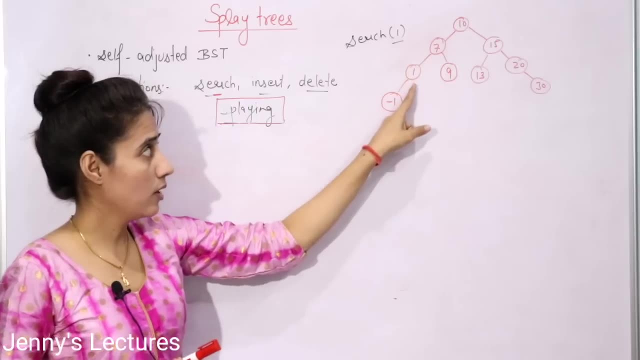 now the same step. first of all, perform the standard bst searching. compare with this: 10: 1 is less than 10. so we are going to go to the left of this less than 7. now to the left of 7, and here we got 1.. now we do what splaying? now? splaying means this one should. 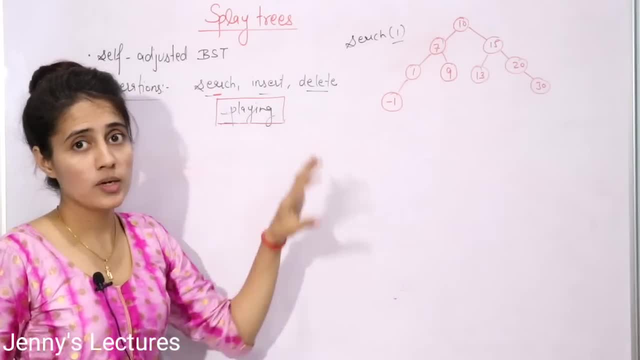 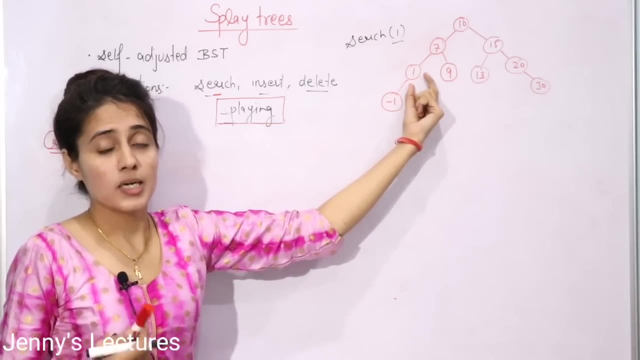 be the root of the tree. you have to make this one as the root of the tree now. you have to rearrange the tree now here. the situation is now this one: this element on which you are going to perform the operation, that is, searching operation, is having parent as well as grandparent right. 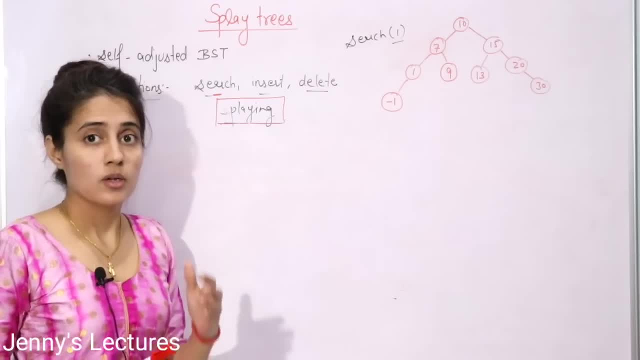 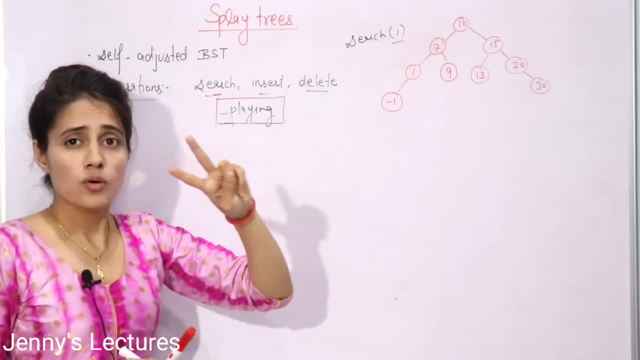 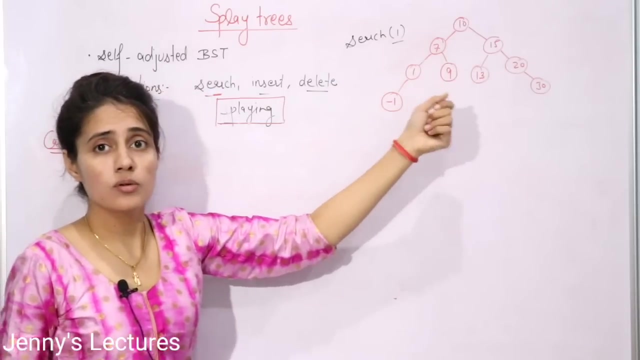 now you cannot do simply zig rotation or zag rotation. now, this is the scenario of zig zig rotation. why so? because here you need two rotations. two in this case you need two right rotation. if you want to search 20, in that case you will- you will need two left rotations. right means zig zig rotation. 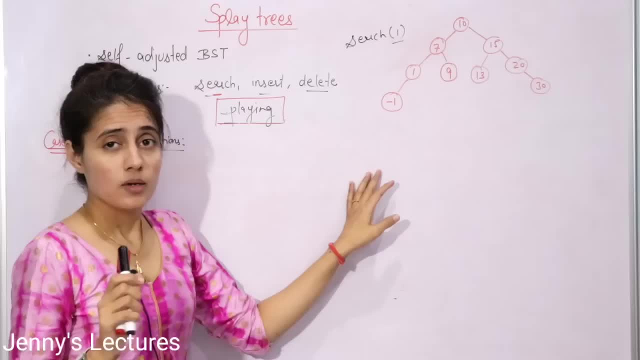 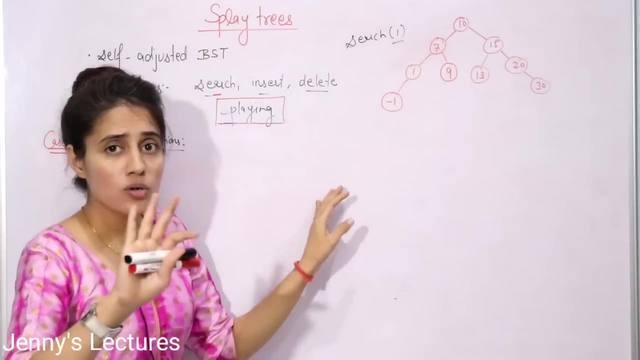 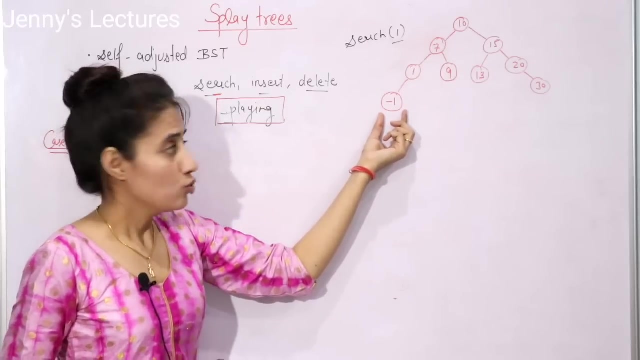 the third case is zig zig rotations. so now, first of all, we perform first zig operation on this 10, then again on this 7.. see, it is not compulsory that the grandparent should be root here. maybe a case that here i want to search minus 1.. so minus 1 is having parent 1 and grandparent 7.. 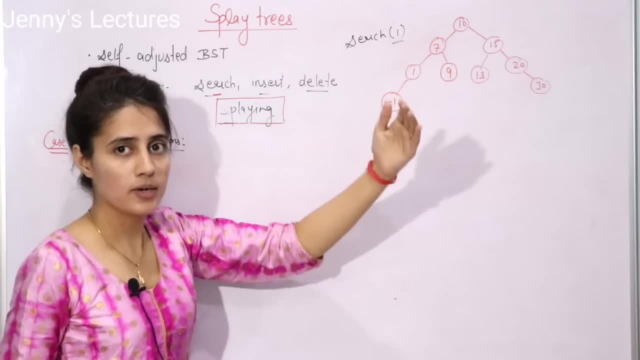 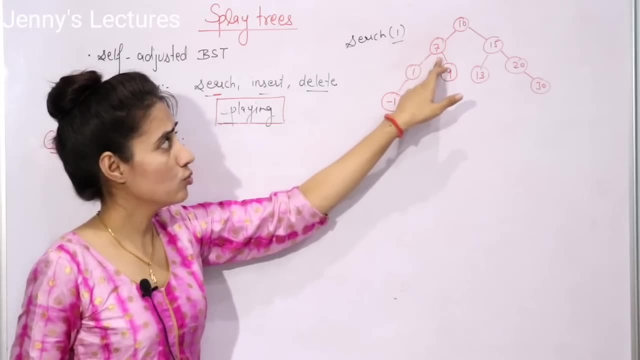 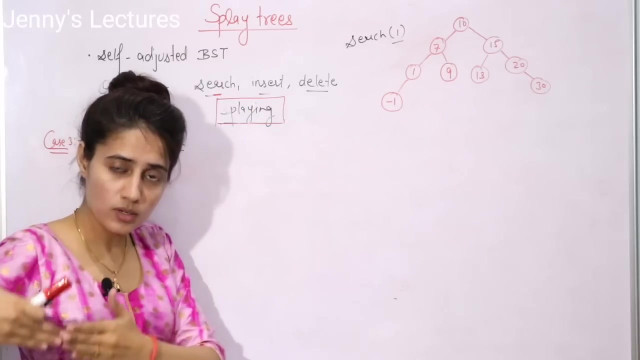 seven. this thing you need to take care. just find out: parent, grandparent. if this is the case, now find out which rotation you need. both are: this is to the left of parent and this is to the left of its parent means zigzag rotations. in same way, if both the the item you want to search and the 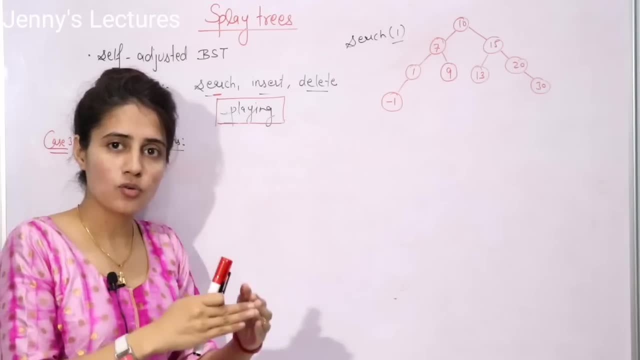 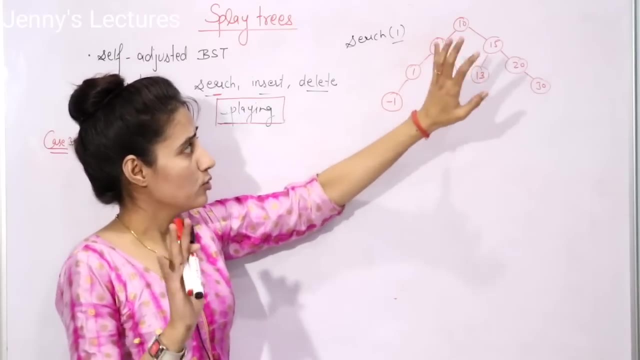 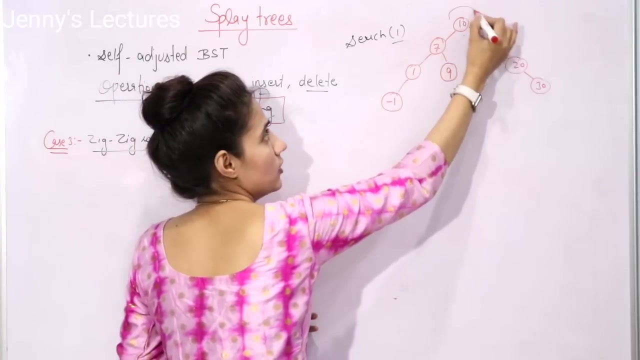 parent of that item is on the same side, then zigzag rotation. it can be either left side or right side. fine, now here. here suppose i am taking a case, i am searching one now. first of all, we will do: zig rotation on this 10 means first right rotation on this 10. we are going to pull this. 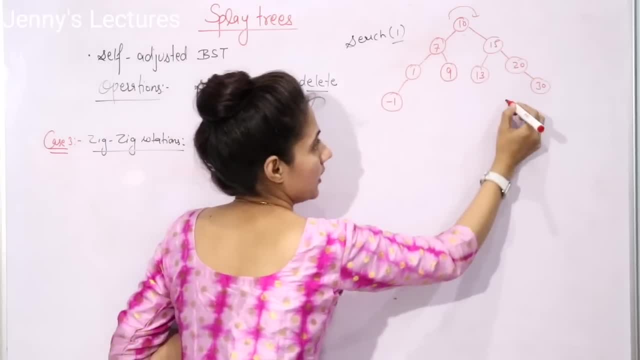 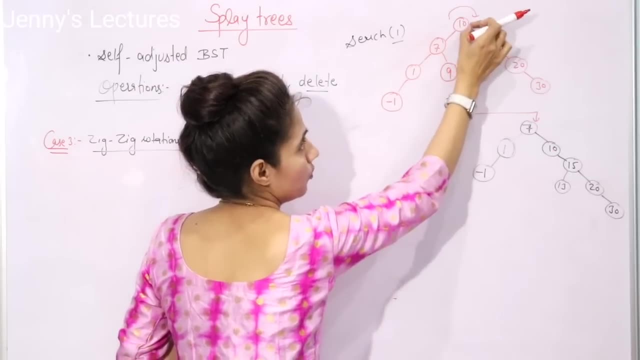 10 downward and 7 would go upward. now the tree would be something like this: see here, the 9 is to the right of this 7. now to the right of 7 we have. after pulling down this 10, we have 10, so 9. 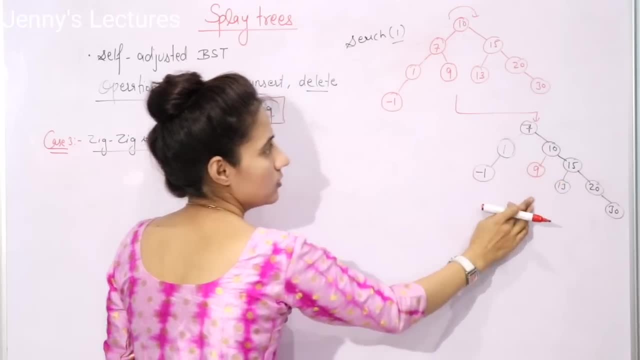 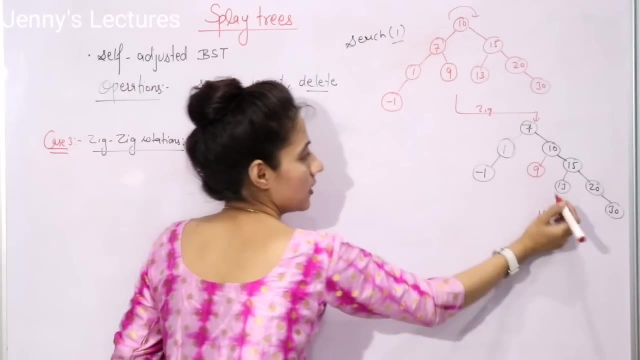 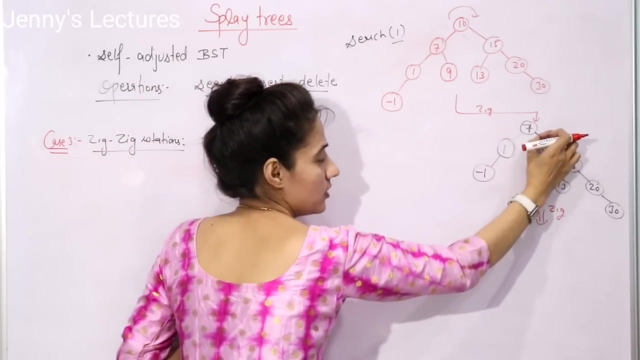 would go to the left of this, you 10. so now this is the tree. after one rotation, now again we will perform zig rotation. this is one zig, this is again zig. that is why it is known as zig zig rotation. now again right, right rotation on the 7: 7 would go downward and now one would go upward. so now the tree would be something like this: 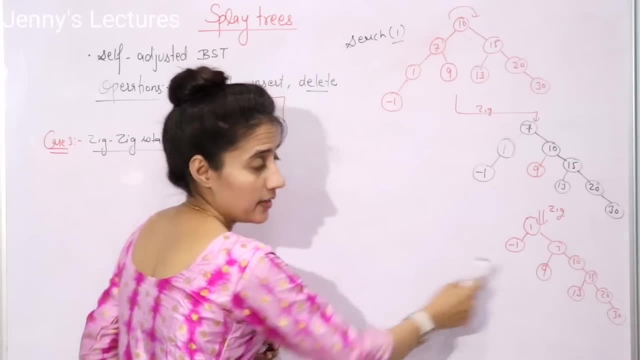 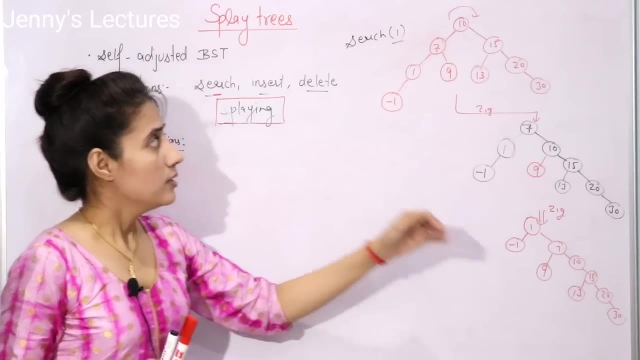 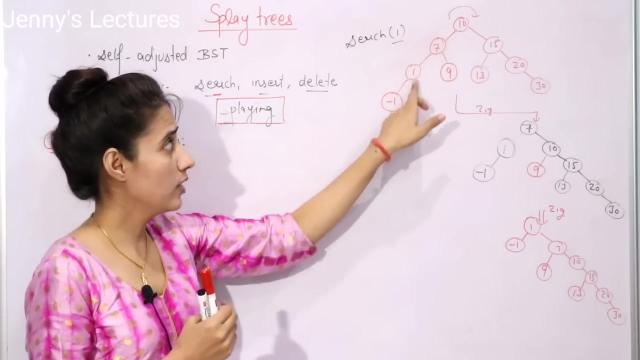 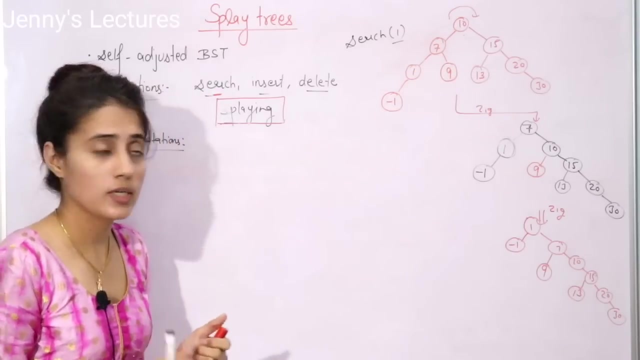 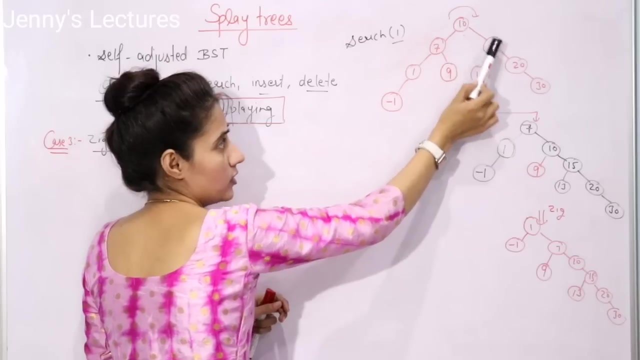 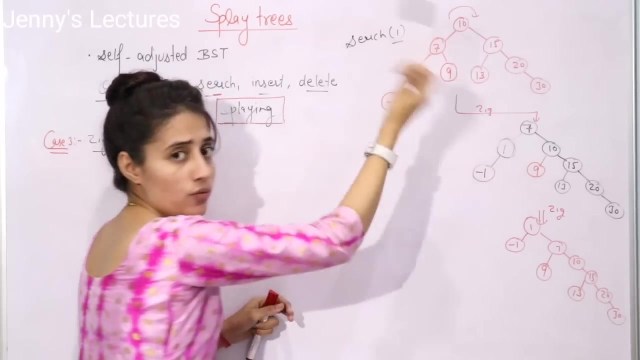 so now this is the final tree here you can see one is now root of the tree. now we are done with searching right now. see again. the symmetrical case of this may be: these are to the left of its see, one is to the left of its parent and 7 is also left of its parent. now suppose i am taking a case. i want to search 20 now find out where is 20, start with the root, greater than 10. so we are going to the. we are going to search in the right side of this, 10 greater than 15. here we got 20. now see 20 is having parent and 20 is to the right of its parent, as well, as 20 is to the left of its parent. now see again. the symmetrical case of this may be: these are to the left of its see, one is to the left of its parent and 7 is also left of its parent. now suppose i am taking a case. i want to search 20 now find out where is 20, start with the root greater than 10. so we are going to the. we are going to search in the right side of this, 10 greater than 15. here we got 20. now see 20 is having parent and 20 is to the right of its parent, as well as 20 is to the left of its parent. now see: 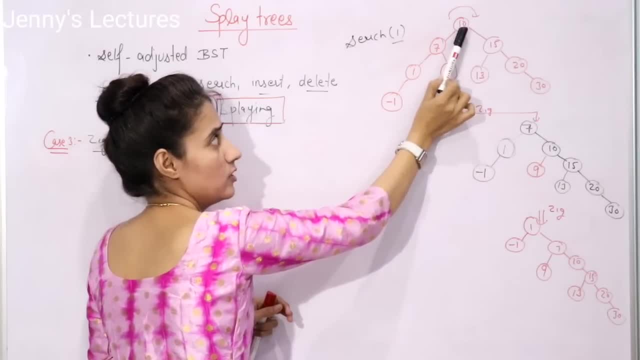 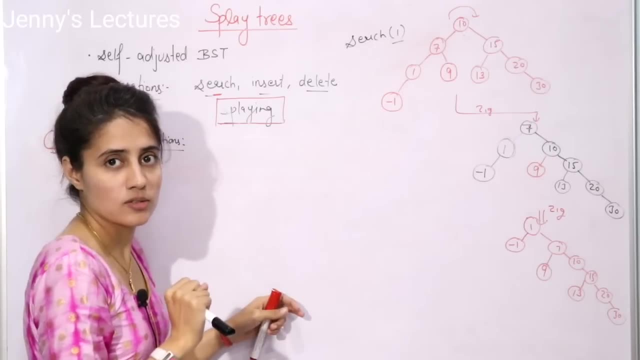 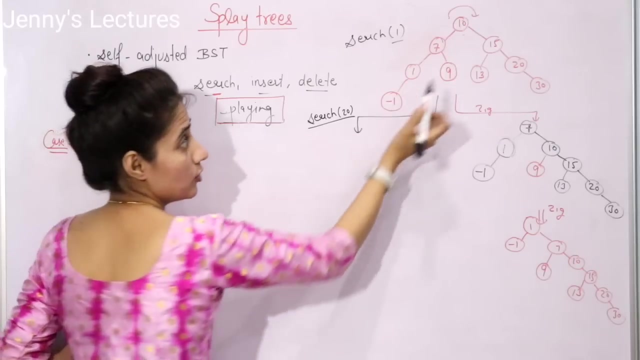 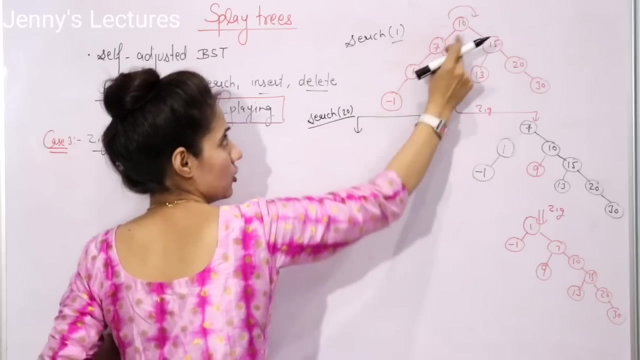 having grandparent, and this is also this. 15 is also to the right of its parent. means here we know we need what- two left rotations, right. so now the tree would be something like this: after two left rotations, so now, first of all, the left rotation on this 10 right, then again left rotation on 15. so after doing the first left rotation on 10, the tree would be something like this: see this: 13 is to the left of its parent as well as 20 is to the right of its parent. means here we know we need what? two left rotations, right. so now the tree would be something like this: after two left rotations, so now, first of all, the left rotation on this 10 right, then again left rotation on 15. so after doing the first left rotation on 10, the tree would be something like this: see this: 13 is to the left of. 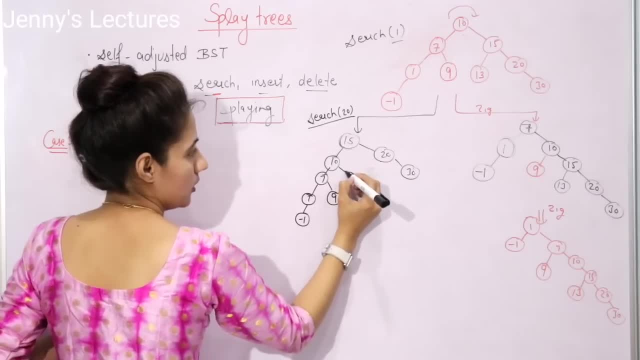 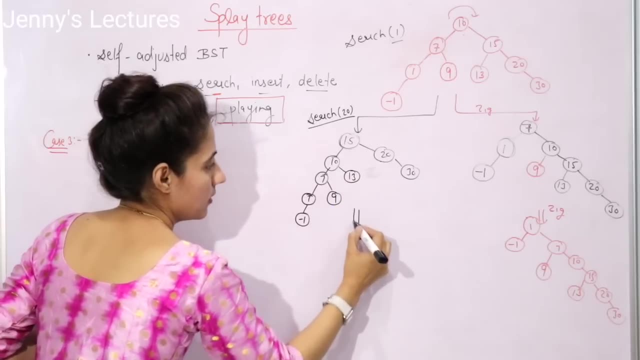 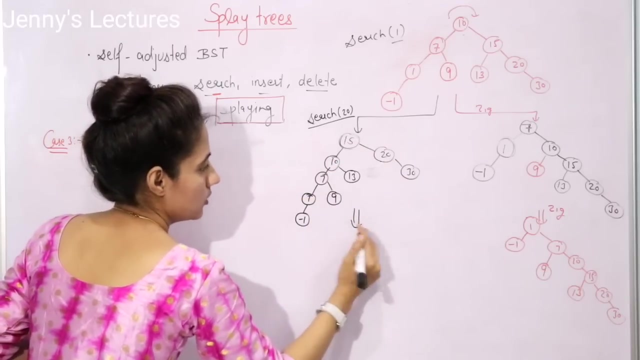 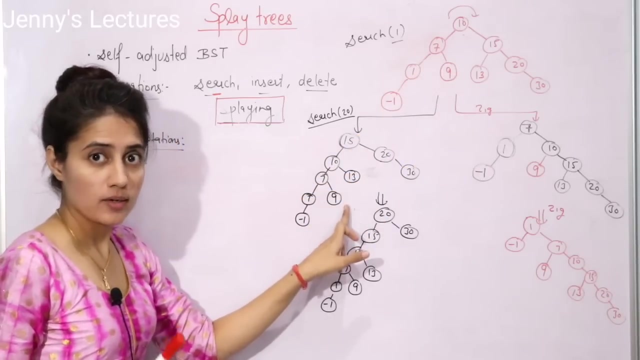 15 means to the left of 15, so here to the, it will come to the right of this 10. so now here we got 13.. after one left rotation, now again second left rotation. we will pull again 15 downwards and 20 would go upwards. so now the tree would be something like this: so now this zigzag rotation is having two cases: one, is this one, this one, and second, is this one right, this? you can say that it is zigzag right rotation. it is what. 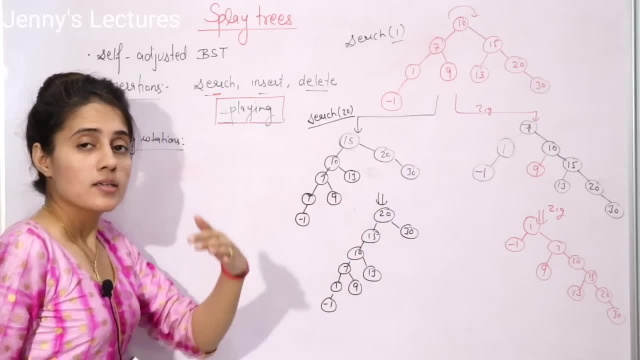 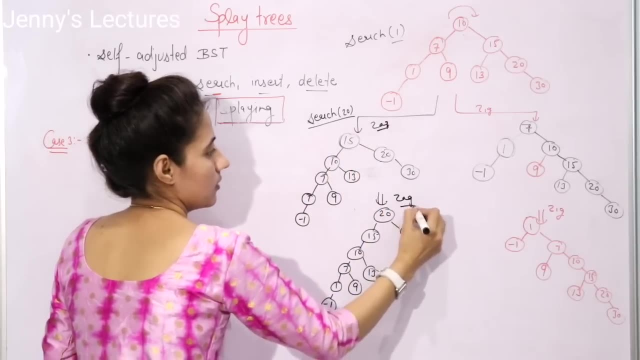 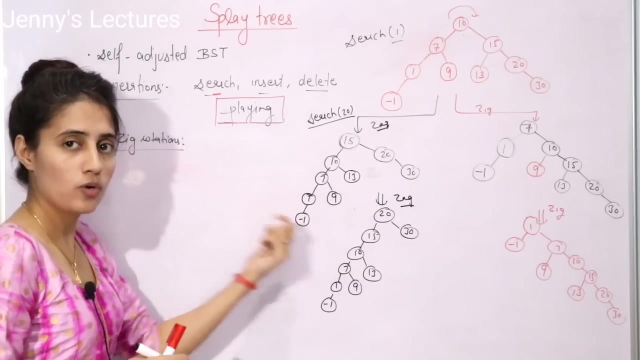 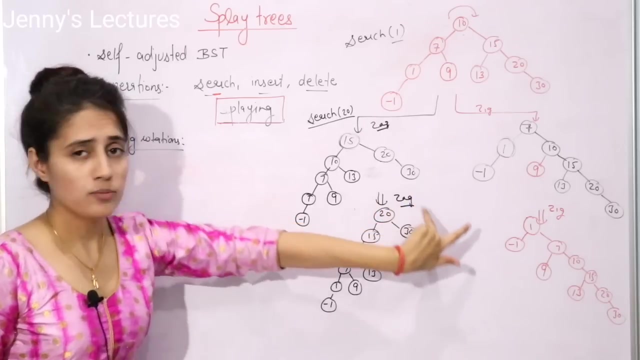 zigzag, left, left rotations, and somewhere it is written that it is what? zig rotation? first zig rotation and again zig rotation. because zig we have already discussed in this video- only that it is when you are going to do left rotation, then that is known as zig rotation. right rotation means zig rotation. so here, if you write these are two types of rotations. 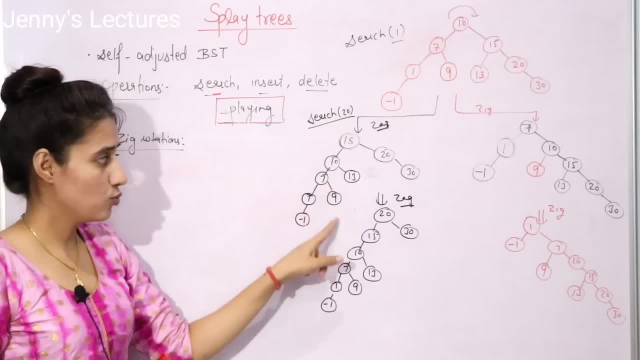 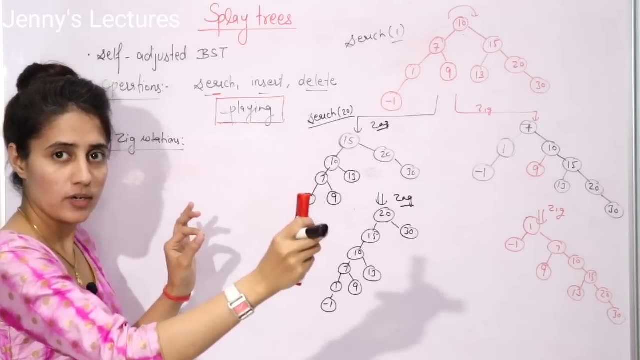 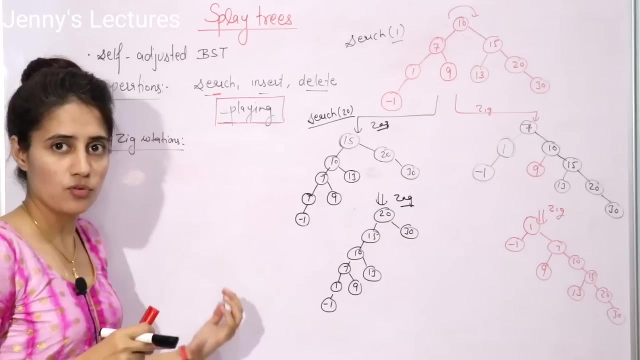 zigzag means this one, this example you can take. zigzag means this one, this example you can take. that is also right. and if you write in one simple step, that is zigzag rotations, fine. so in that case only you can give these two examples: this is zigzag, right. this is zigzag left rotation, fine. 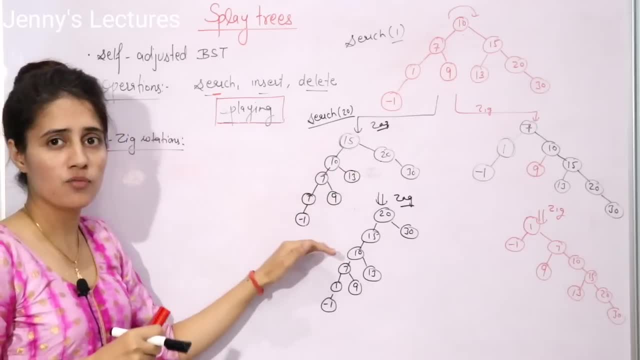 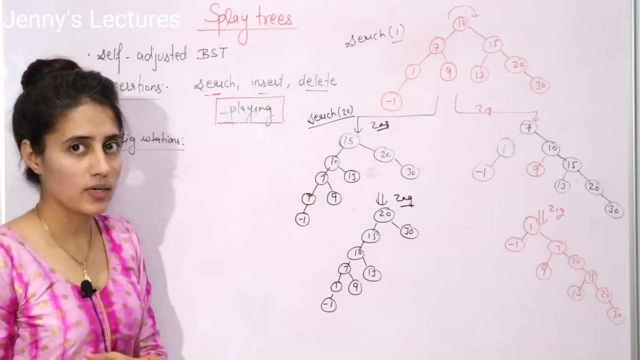 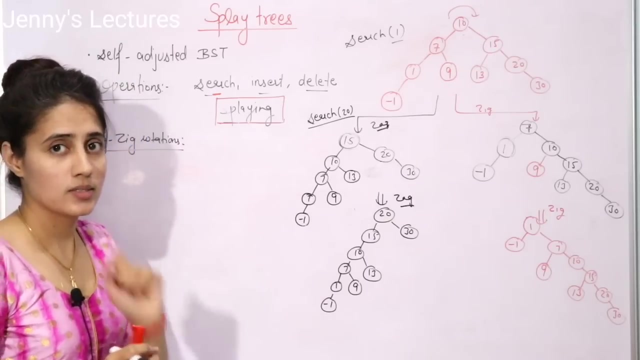 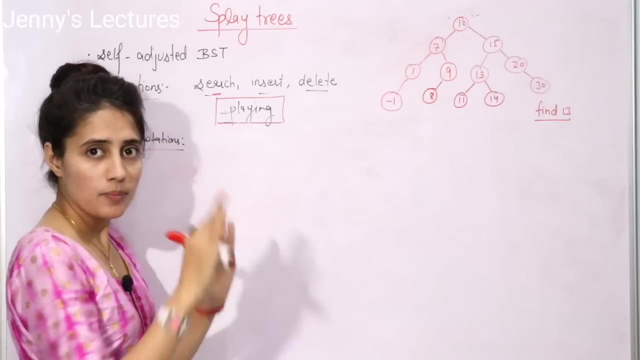 both are correct. somewhere you will find this is zigzag, somewhere you will find these two cases are example of only zigzag rotations. so don't get confused: both are correct right now. next next situation may be a zigzag situation. now what is that thing? see? now let us take this example, and here i want to find 13, or you can say search 13.. simple bst. 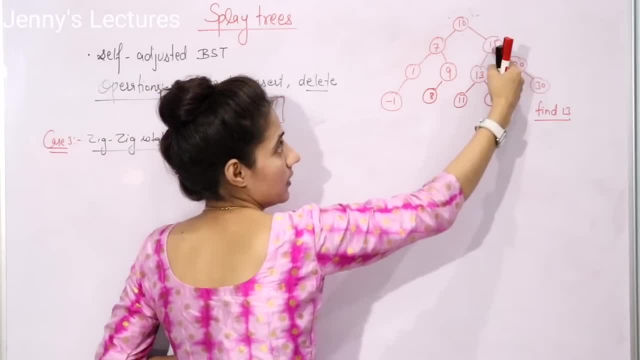 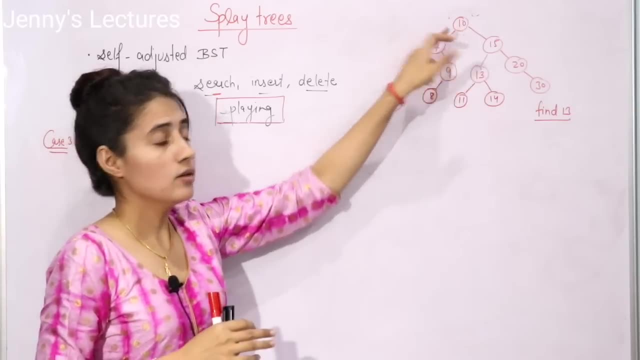 searching. compare with this: 10 greater than 10, less than 15. here we got 13 right, so now see now splaying 13. you have to make this 13 as a root of this tree. now see 13 is what to the left of 15. 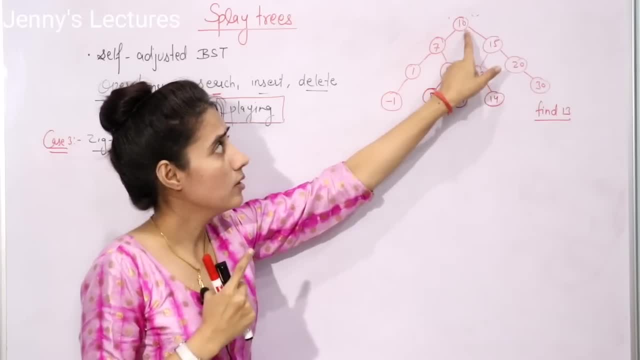 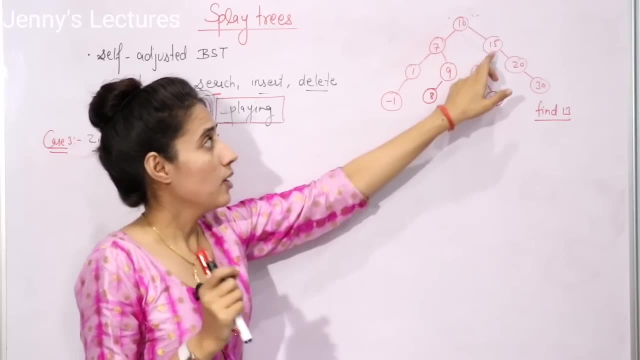 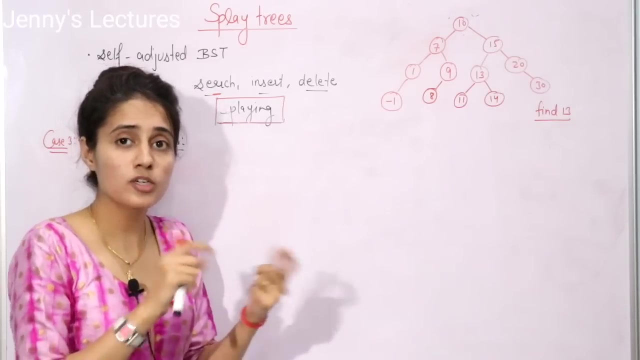 to the left of its parent and this 15 is to the right of its parent. this is see this 13 is having parent as well as grandparent. fine, but now parent is now this is to the left of parent, but this is to the right of this case means left right situation is there. so it is what zigzag situation. 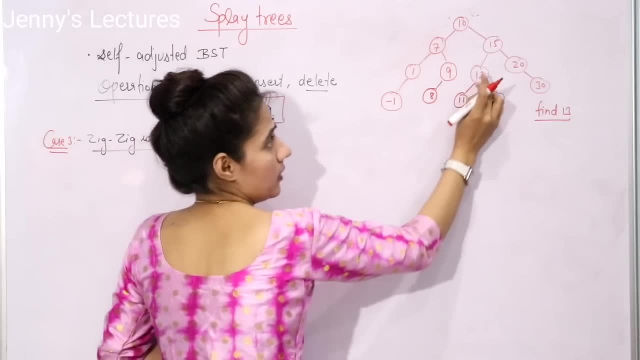 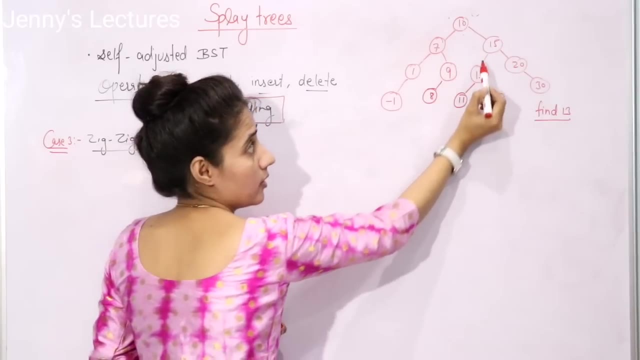 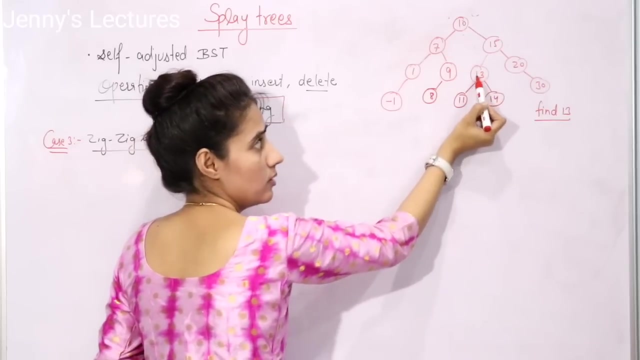 see how this is zigzag situation. first of all, this 13 is to the left of this 15, so we will do right rotation right. when you do right rotation on 15, on this edge, which is connecting 13 and this 15 means the node you want to search and its parent, first of all, you will do rotation on that edge. you are not. 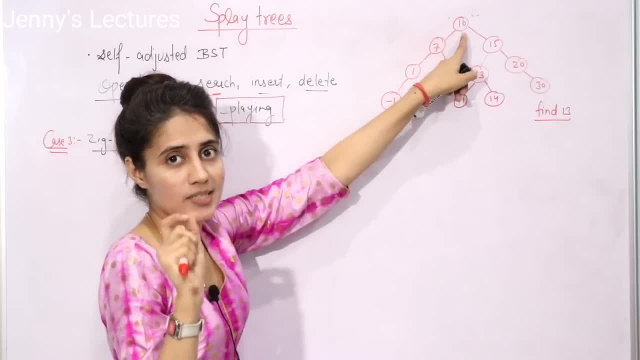 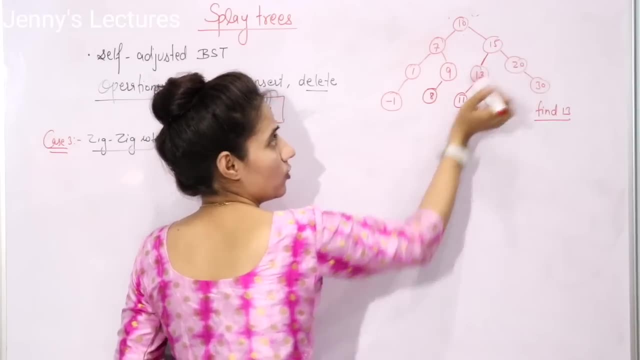 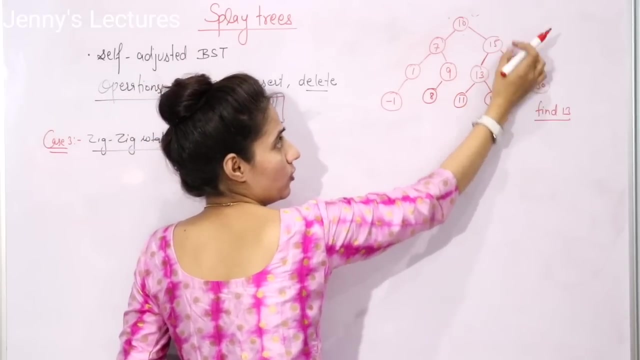 going to do rotation on this: 10 now right in zigzag situation. first of all, we will rotate this on this edge. so on this you are going to do right rotation right means zig rotation. now 13 would go, we will do right. rotation means 15 would go downward, 13 would go here now to make 13 as a. 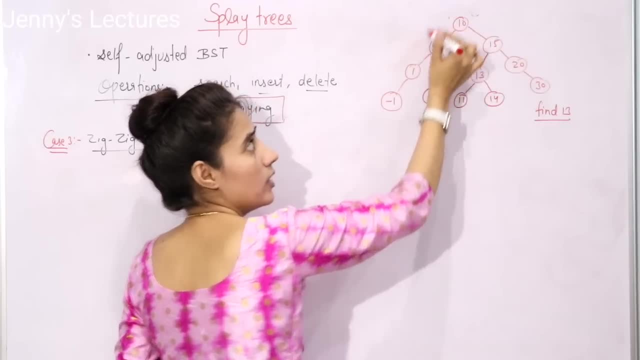 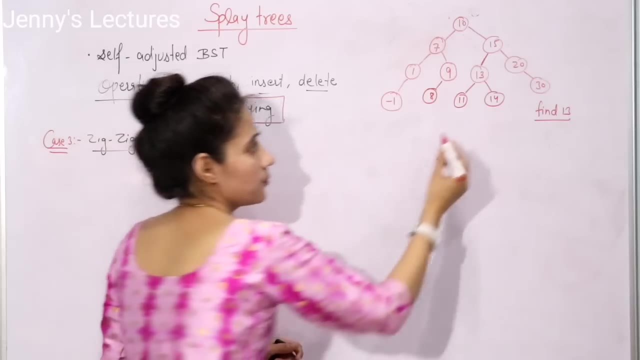 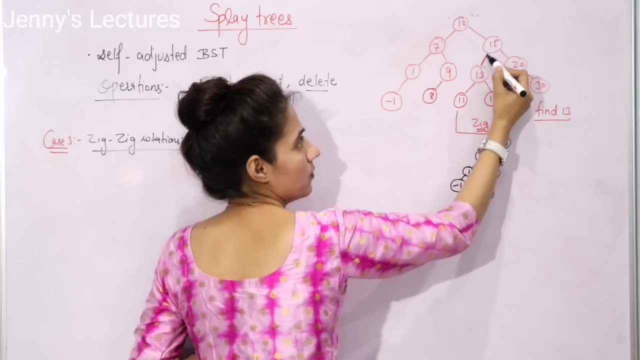 root, now 13, is to the right of 10, we will do left rotation. left means zig rotation. that is why it is known as zigzag rotation. right now. see, first we are going to perform zig rotation, so now the tree would be something like this: zig rotation on this edge means zig rotation on 15 to the, on the parent. 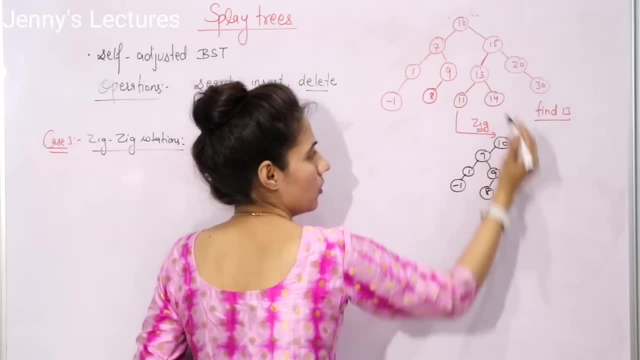 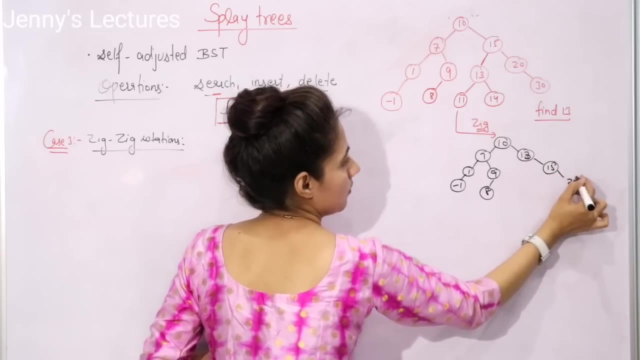 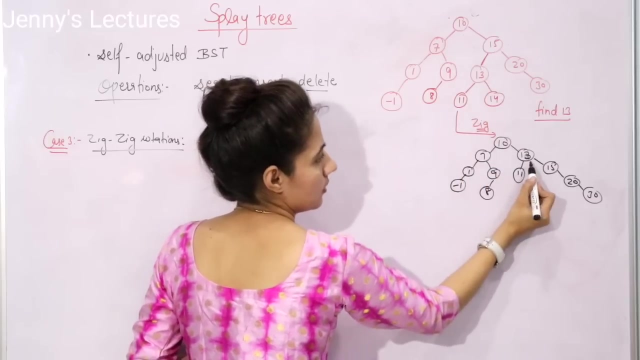 of this node. so 15 would go downward, 13 would go upward. now here we have 13, 15. to the left of 13 we have 11, and to the right of 13 we have 14, means to the right of 13, but now to the left of 15, the 14 would go to the left of. 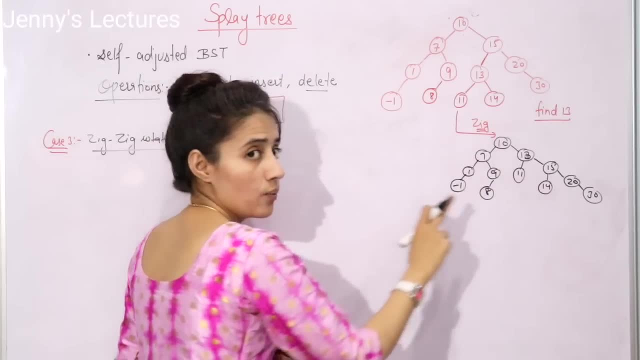 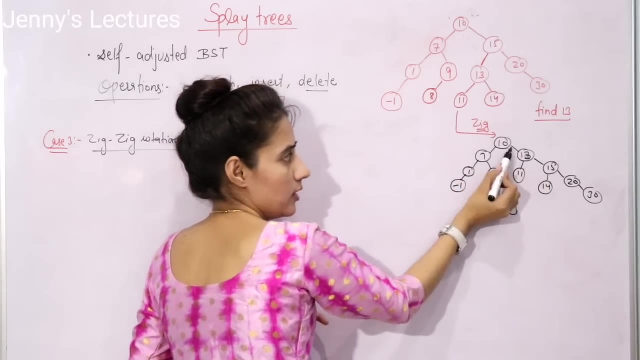 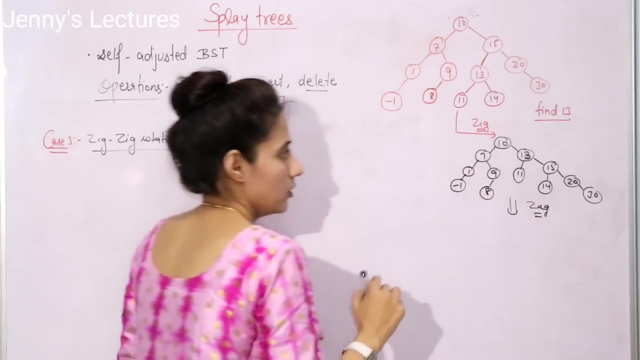 14.. now this is the tree after one zig operation. now, still, we are left. now, still the 13 is not the root right now. now we will do what the 13 is to the right of its parent. now we will do. left rotation means zig rotation. so now, after left rotation on this 10, the tree would be something. 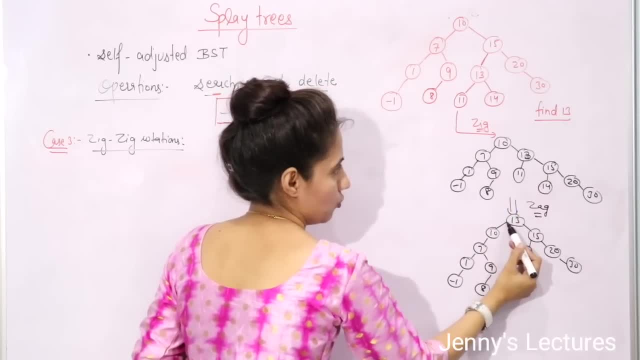 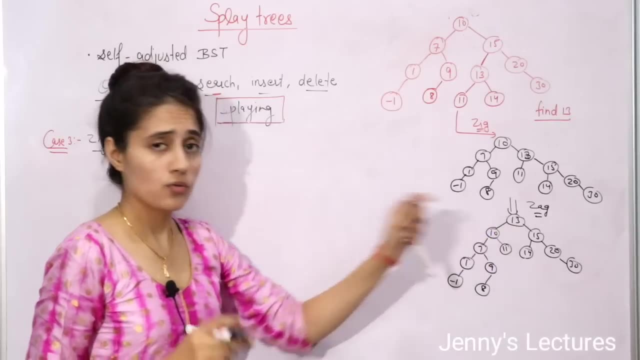 like this: see: this 11 is to the left of 13, so to the left of 13. now we have 10, so the 11 would go to the right of this 10.. now, this is the final tree. as you can see, 13 is now the root, so this is the. 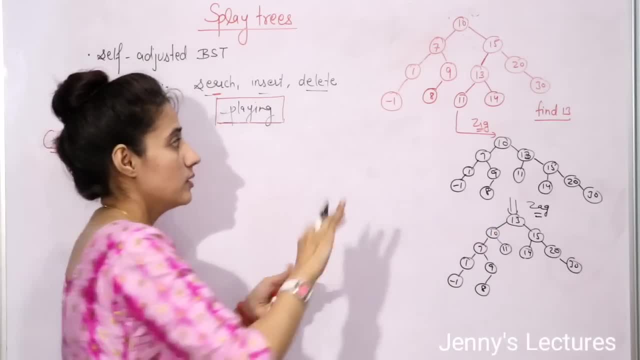 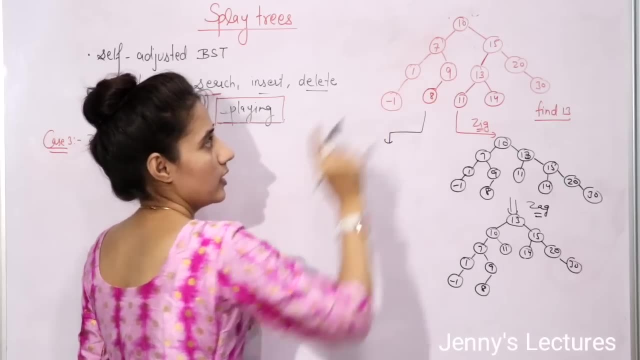 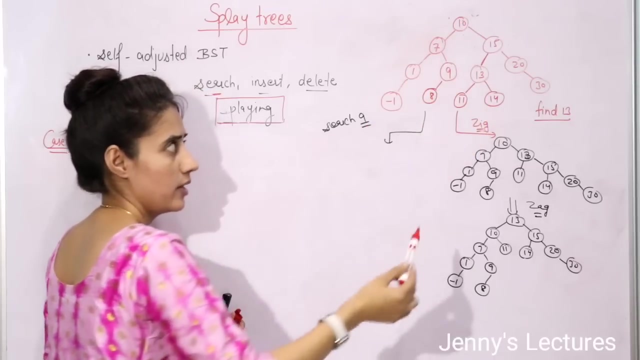 situation, of zigzag situation now. so the second case in zigzag situation may be: what suppose i want to search? 9, now same. compare with this: 10 less than 10. so here greater than 7. so here we got this 9, now we are going to. 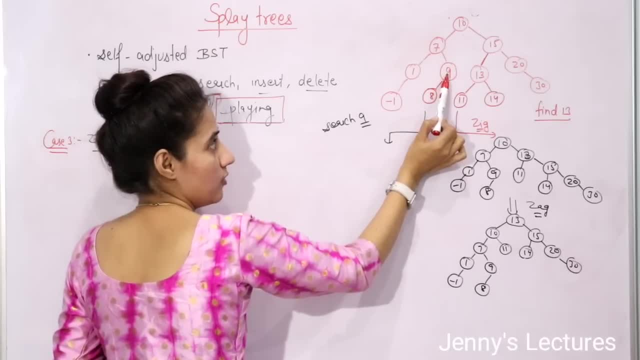 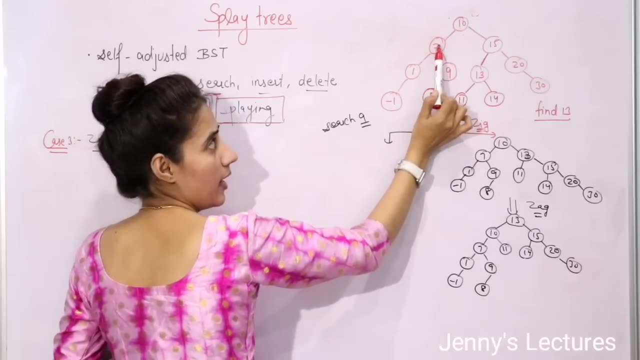 do splaying. splaying on this 9 means 9. we are going to make this 9 as the root of the tree. now see, this 9 is what to the right of its parent and this 7 is what to the left of its parent. right, 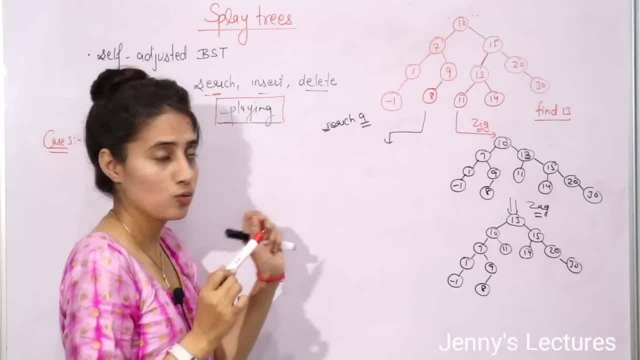 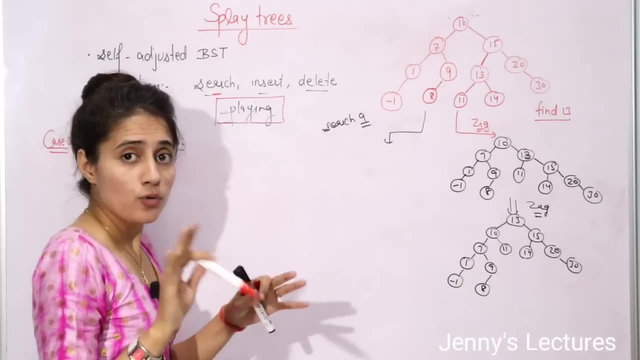 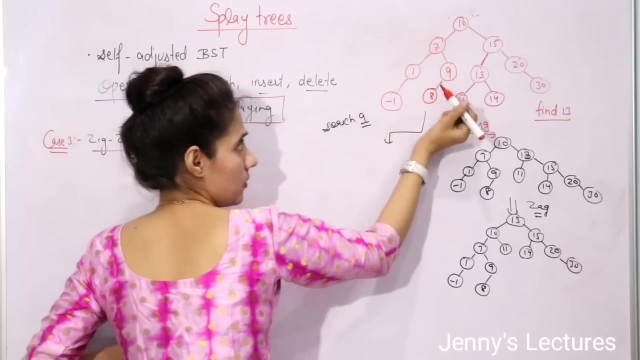 9 is having both parent and grandparent. so this is what opposite to this case. but this is also a zigzag situation now here, or you can say: this is what a zigzag situation. both are correct right now here. what you will do first of all. first of all, we will do what on this edge see this 9 is: 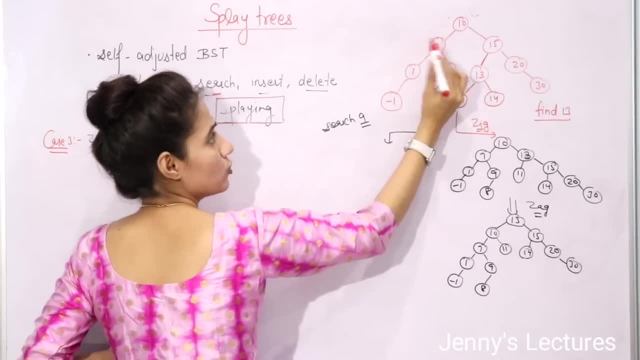 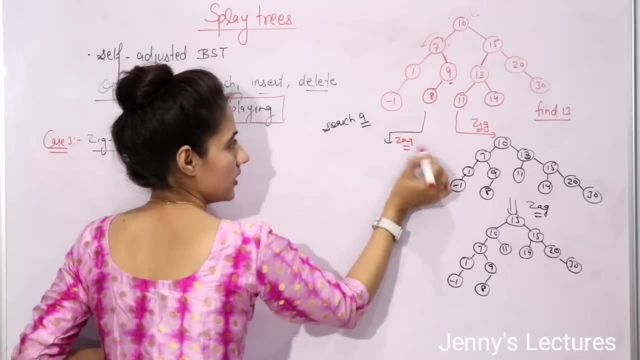 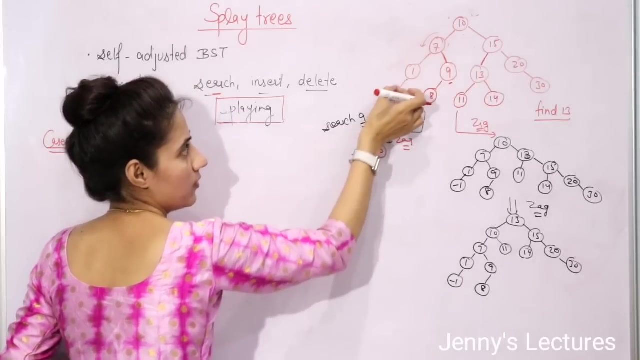 what i want to search: 9. so 9 is to the right of the 7. so first of all we will do left rotation. left means z z rotation, so suppose here i am taking what writing: zig rotation. so after one left rotation the tree would be something like this: root would be as it is. now we are going to pull the 7 downward and 9. 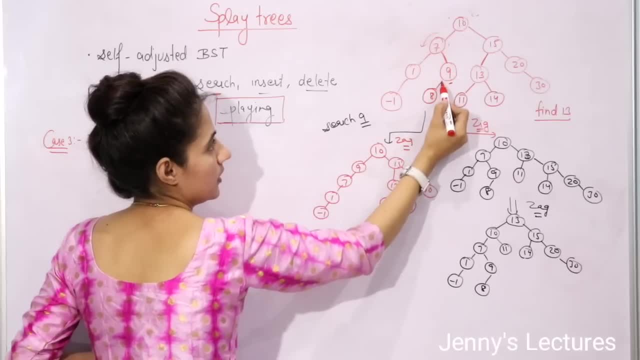 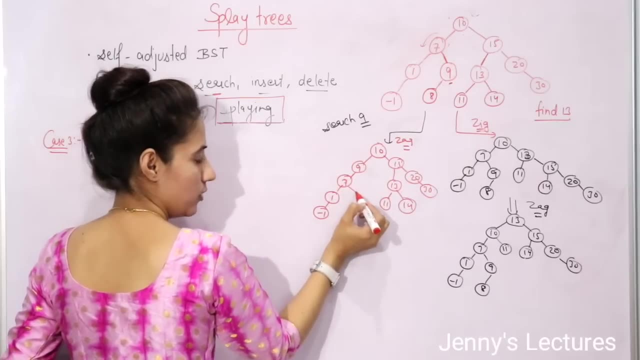 would go upward. so here we have 9. see this, 8 is what? to the left of this 9, so to the left of this 9 is we have 7. now 8 would go to the right of this 7. fine, now again. still, 9 is not the root. so now, 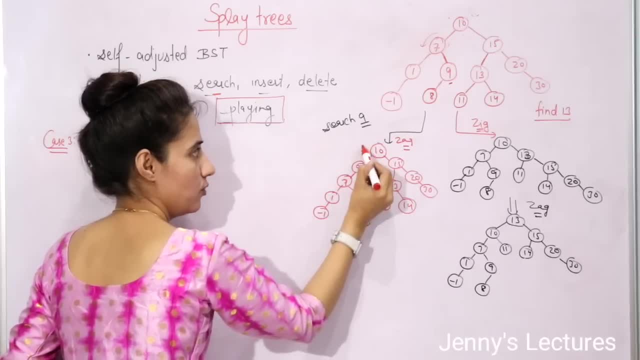 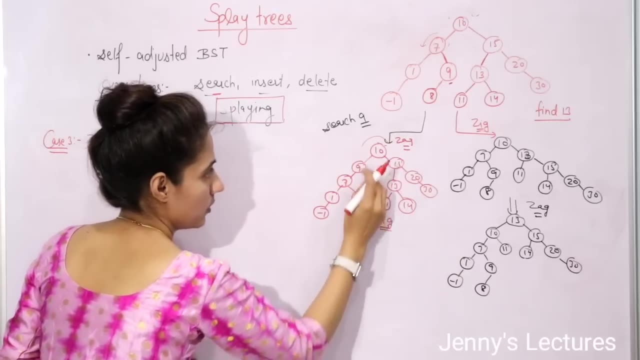 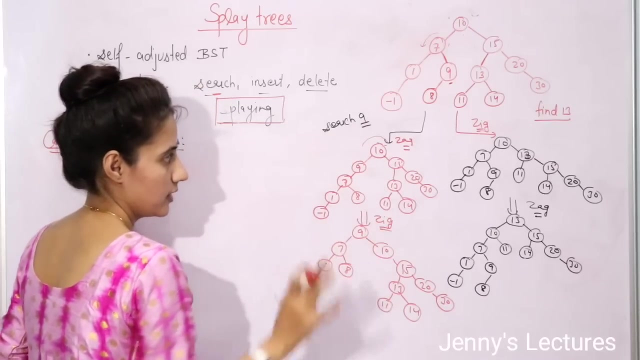 we will do what. now 9 is what to the left of its parent? now we will do right rotations means zig rotation you will do now after one right rotation tree would be something like this: now 9 would go, the root, would become the root. now this is the final tree after zig zig rotation. suppose here we have something to the right of this. 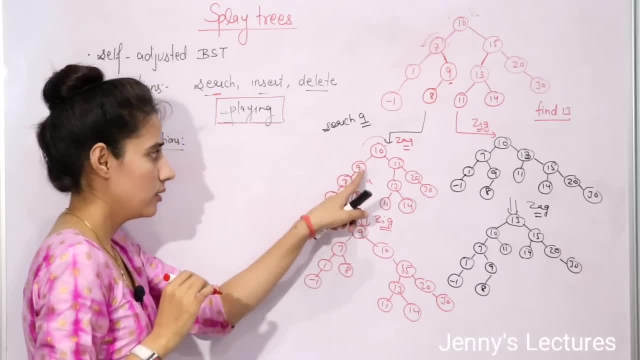 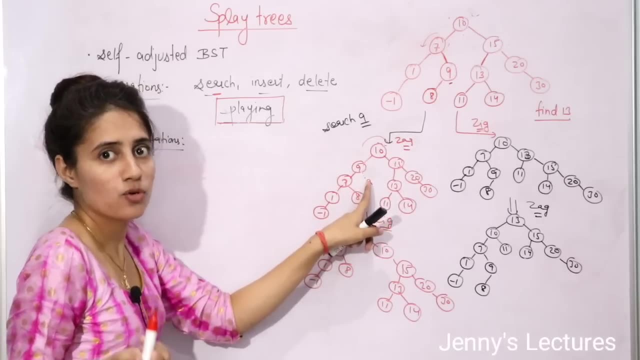 9. suppose i am taking a. we cannot take something here because to the right of 9 the data would be greater than 9 but less than 7. what we can do it is 9.5. you can say right, just for understanding purpose. so here suppose i am taking. 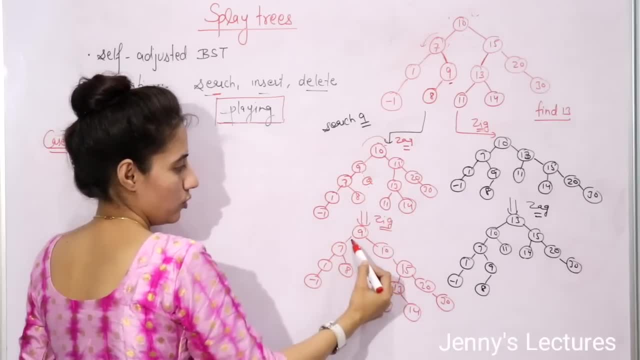 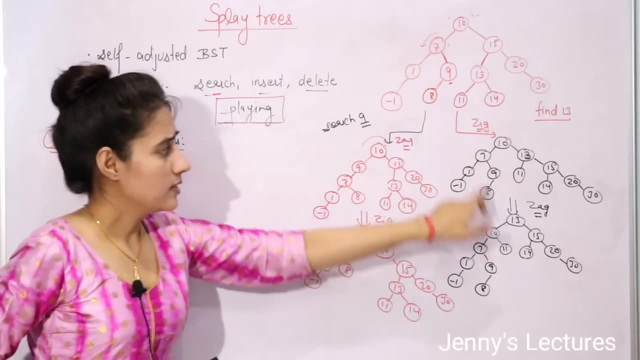 a. so now the a would go- it is right- to the 9, so it would go to the right of the 9 and the left of this 10.. i hope you know this point right. this is what a zigzag situation. this is zig zig situation. 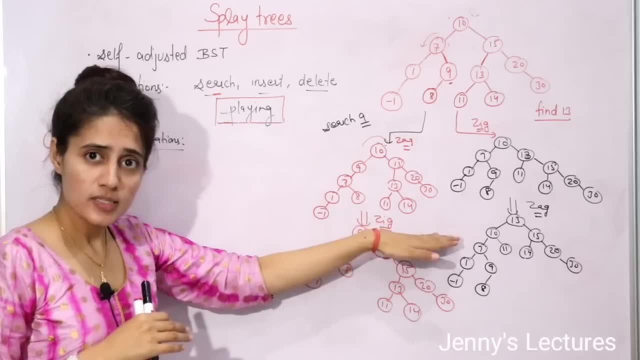 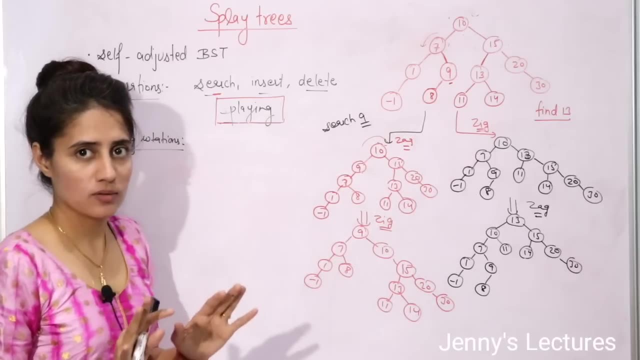 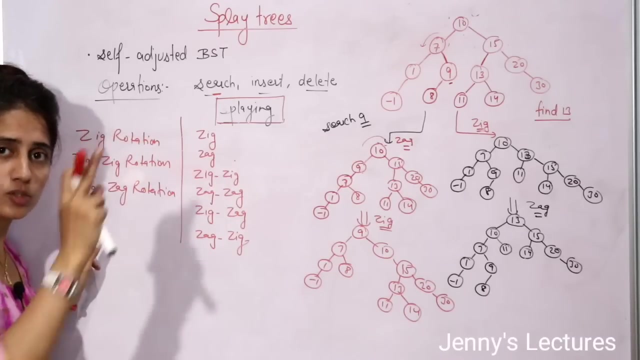 now you can take, you can write down the both the cases means two rotation you can write down or you can take it within one rotation, that is zigzag rotation. so now we have discussed all the rotation. so somewhere you find out that they have written these three rotations only in splaying of. 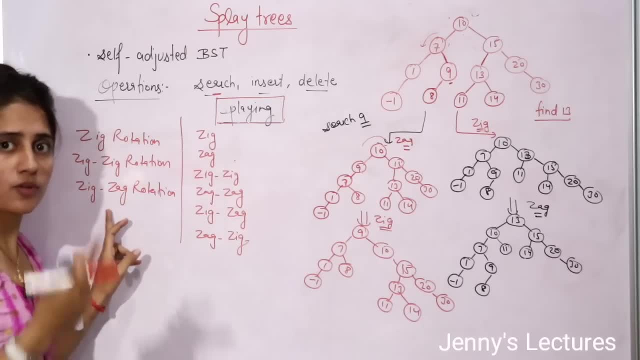 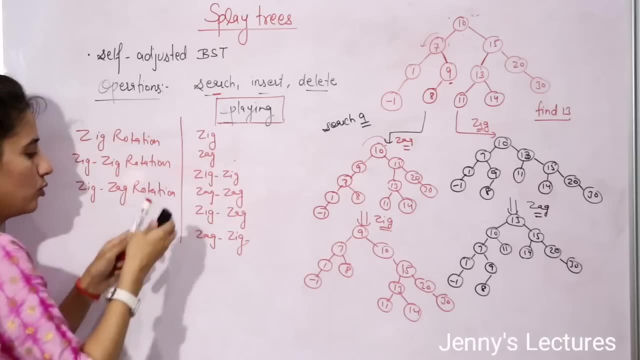 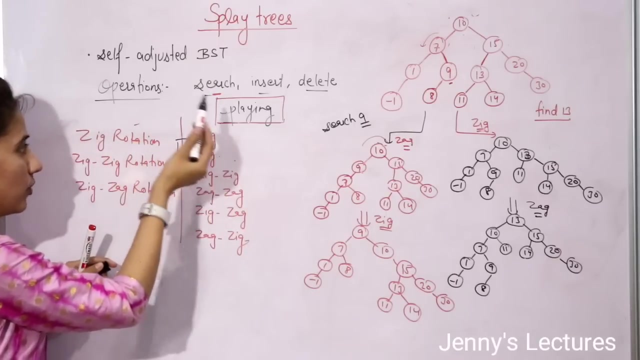 the tree zig rotation, zigzag and zigzag, or somewhere you find out that they have written six rotations. fine, so here in zig rotation they have covered both the cases, zig and zig. right, either you can write down separately or you can write down in one rotation, and in zig, zig rotation they have covered both zigzag and zigzag, and in zigzag rotation they 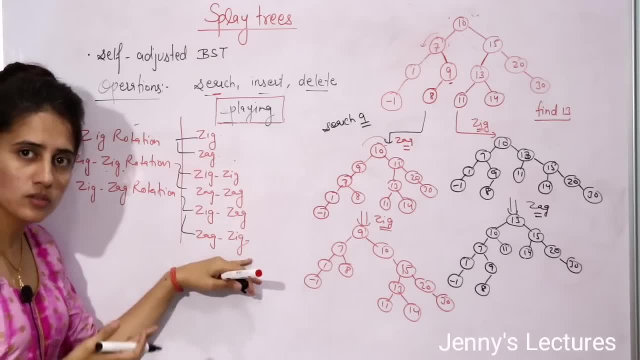 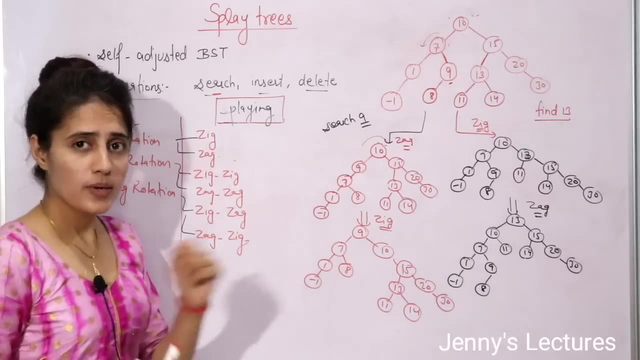 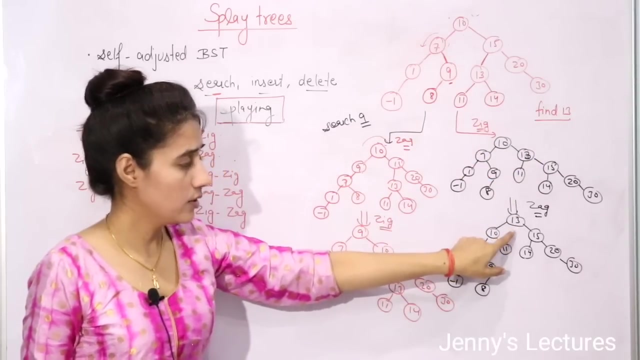 have covered zigzag and zigzag so that you can write down this: six separate, six cases, or within three cases, you can write down all the six cases. now some advantages of split trees or what see here we have done what search 13 right after searching 13 what the tree is, something like. 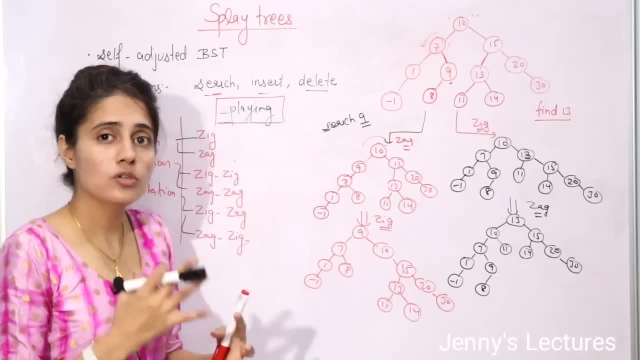 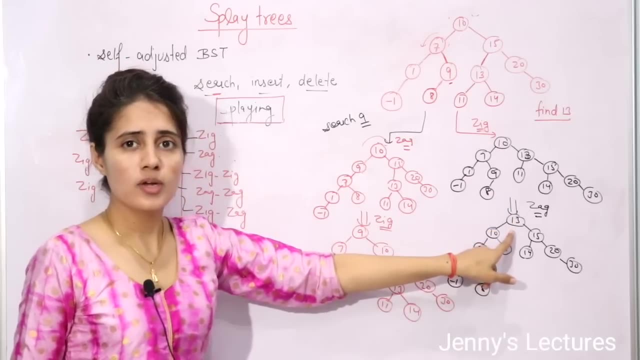 this now. 13 is the root. now suppose again you want to search 13. in that case, how much time you need? only order of one time. complexity, because we are going to compare with the root, and root is only the same tree, sorry, the same node that you want to search. that is 13, so it is going to take order. 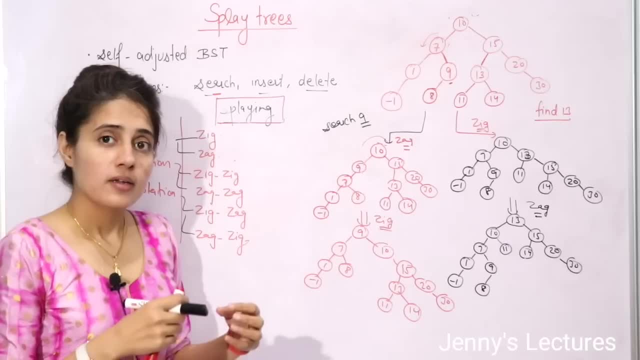 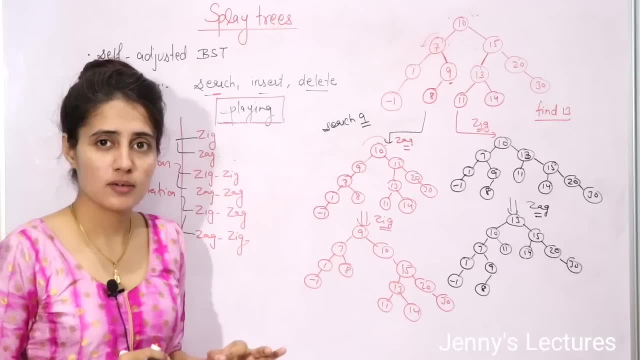 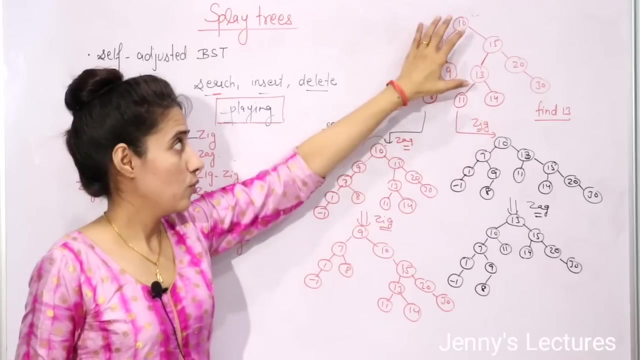 of one time. complexity, right? so now you can say if, in this case, 13 is the frequently accessed, the most frequently accessed element, right? in that case suppose, again and again, again and again, i'm accessing this 13, i'm searching this 13 now at first, once you have searched, 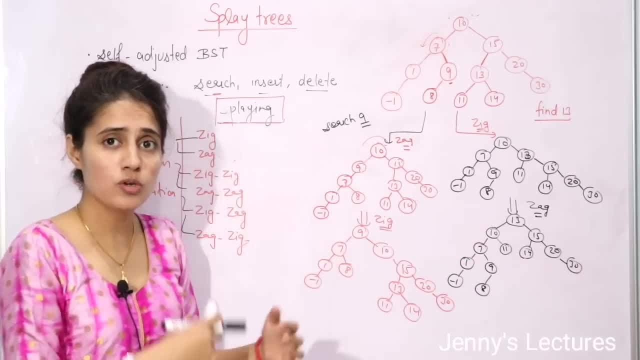 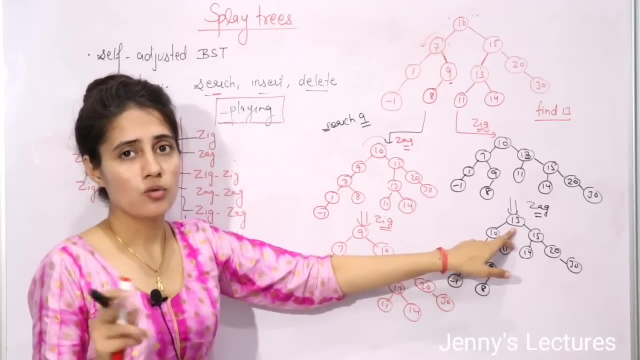 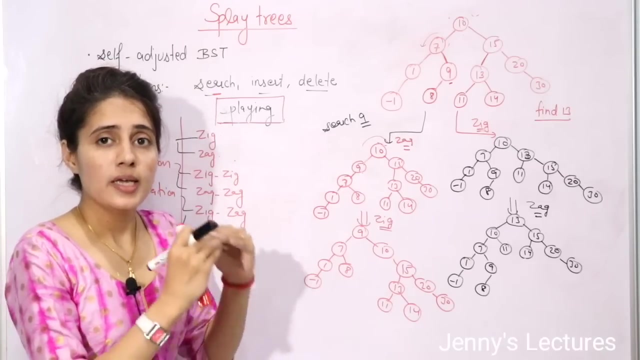 13, now three, something like this. now again, if you suppose five times, you are going to search 13 in a frequent axis. now, 13 is what the root only. you need to take order of one time complexity, right. so that is the main advantage of splay tree, the most frequently accessed element. would be near to the root after splaying the tree. right, i'm saying near to the root. maybe not the root, but near to the root maybe be 10 or 15 is the most frequently accessed element. so 10 is obviously to the near to the. root. only one comparison- you need 15- is also to the near to the root right. so that is the main advantage of splatry: that the most frequently accessed element would be near to the root, so that you need to take less time to search those items. fine, and that is why. because of this, 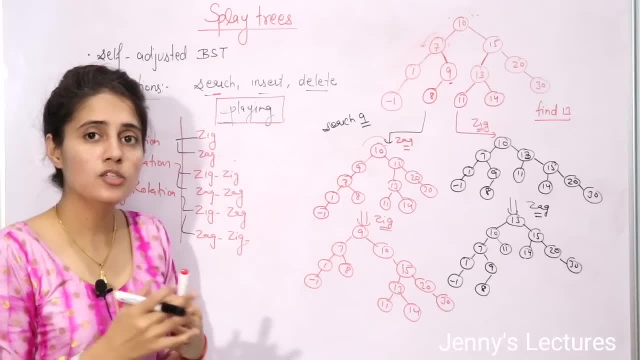 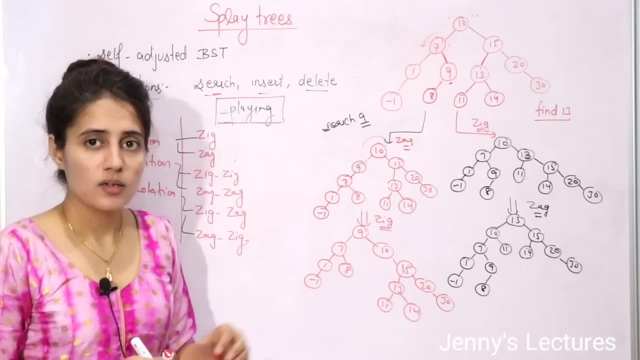 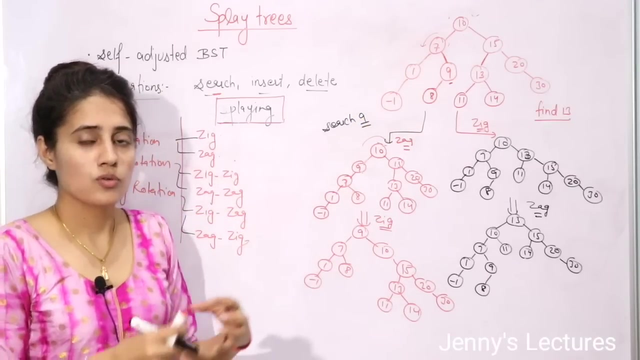 advantage. one application of splatry is what it is used. you know it is better. it is giving better performance in practical scenarios, right, better performance than avl and red black trees in practical situations. so in practical scenarios we are using splatry is mostly right and these 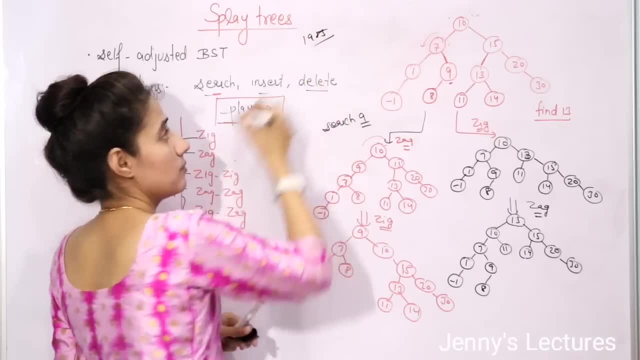 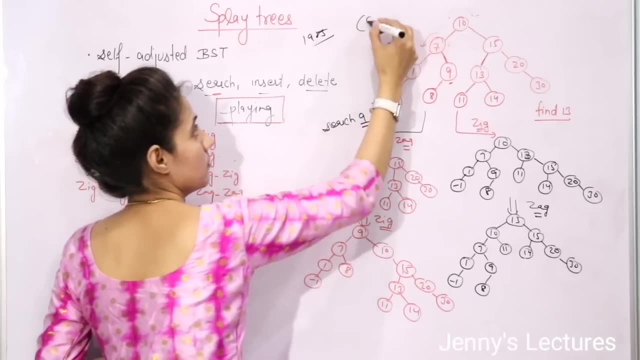 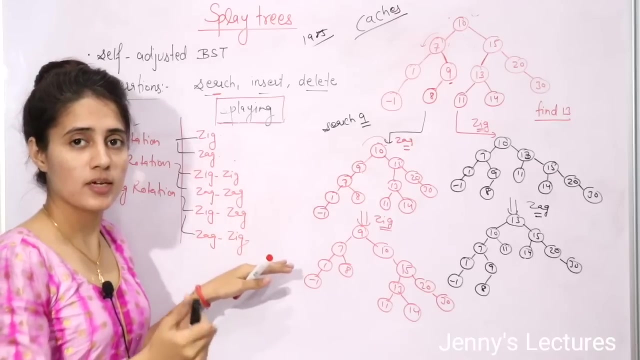 are invented- invented in 1985- fine, so one one application. maybe these are used one application. maybe these are used in 1985- fine, so one one application. maybe these are used to implement caches, right? so i'm going to write down now the advantages, drawbacks and applications. 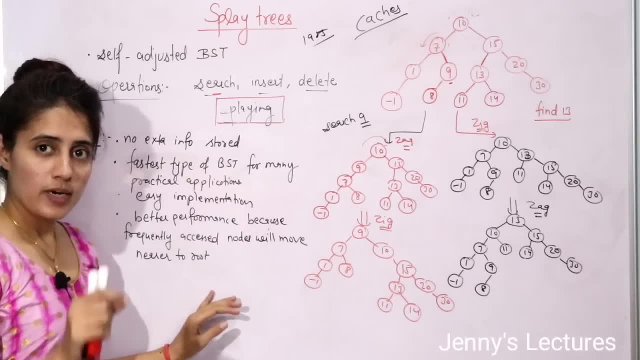 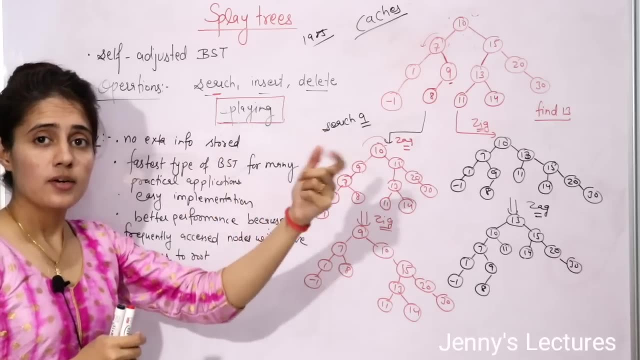 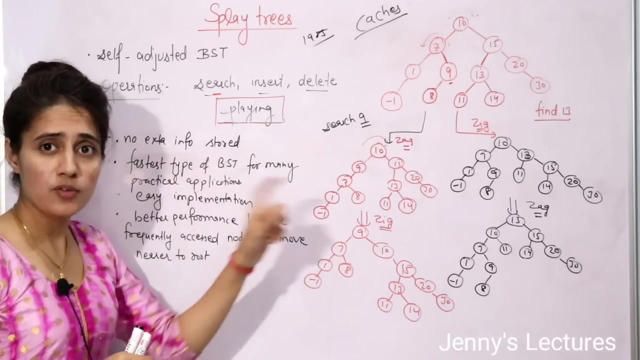 of splay trees. so here are some advantages of splay trees. these are what. obviously these are self-balancing binary search tree, but like avial tree and red black tree, but these are roughly balanced, not strictly balanced, and here no extra information is going to be stored in avial tree. 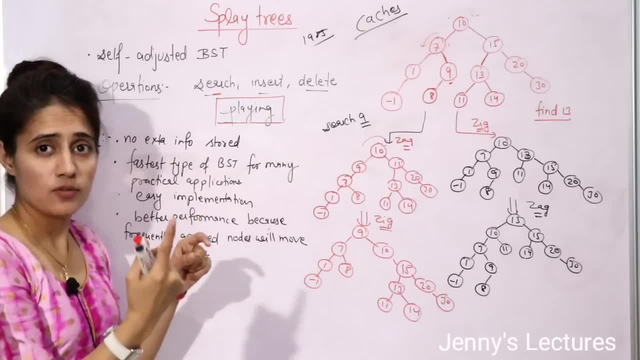 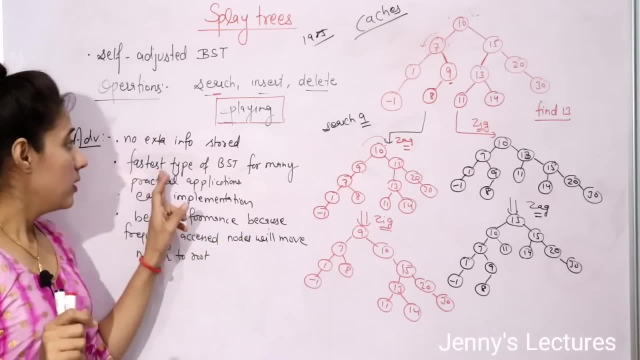 we are going to store what? the difference of what the balance factor we are going to store with each node in red black tree we are going to store the color of the node, but here, no extra information we are going to store. fine, these are, you can see, the fastest type of binary search tree and 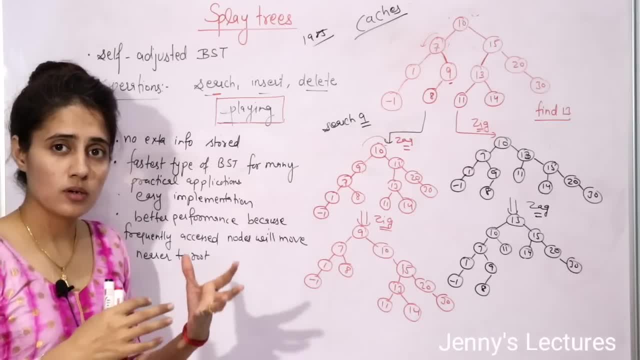 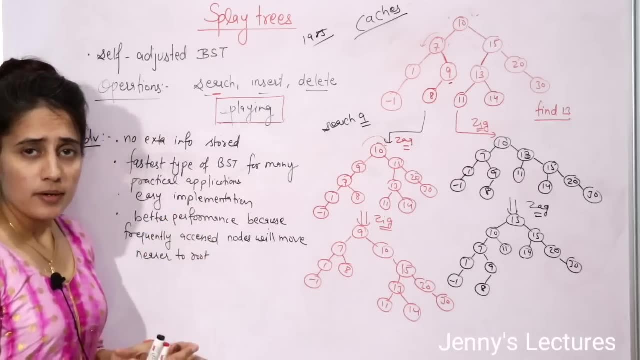 very useful in many practical applications. these are used in windows nt, in gcc compilers right now. these are easy to implement and next may be better performance. this thing we have already discussed with the example. why so? because you can see that in avial tree we are going to store the color of the node, but here no extra. 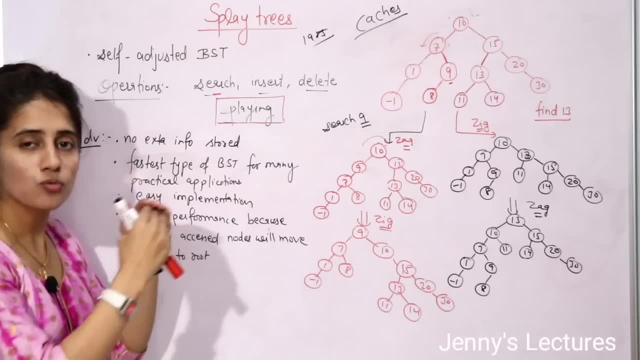 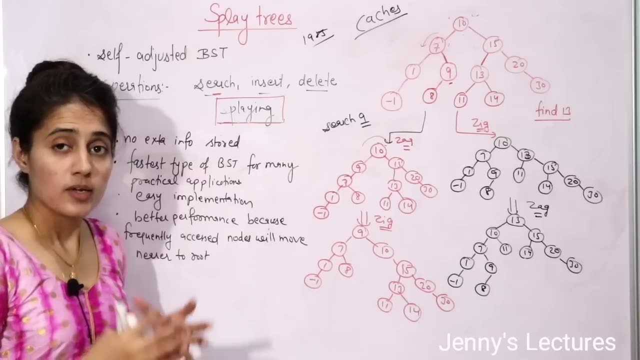 information is going to be stored in avial tree. we are going to store the color of the node, but here frequently accessed elements will move nearer to the root node and we can access those elements quickly right in splay trees. fine, that is why these are going to going to be used in implementation of caches. what is the the principle of cache memory? the most frequently accessed data is stored in caches so that we can to access that data. we need less time, we don't go to the memory to access those data, just we can access that data from the cache, right. so that is why these are used in implementation. 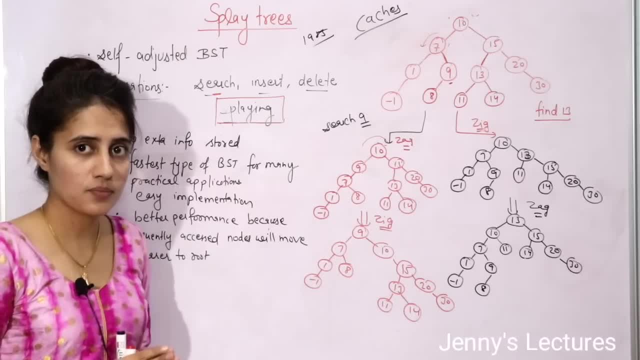 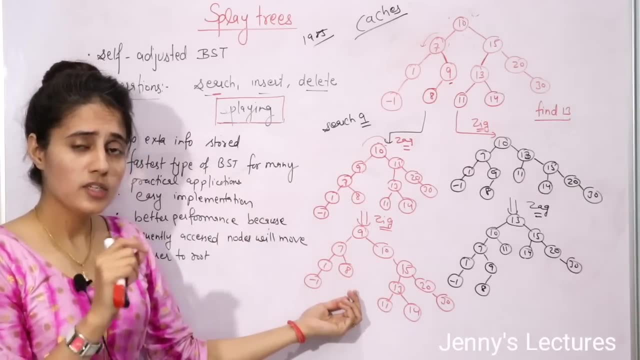 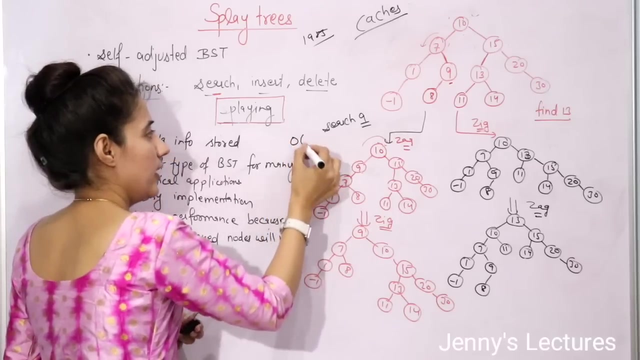 of cache memories to save the time for accessing the data right now. drawback of this tree may be: see one main topic is what. these are not strictly balanced so sometimes the height may be linear or you can say order of n. that is the main drawback of this tree because these are not strictly 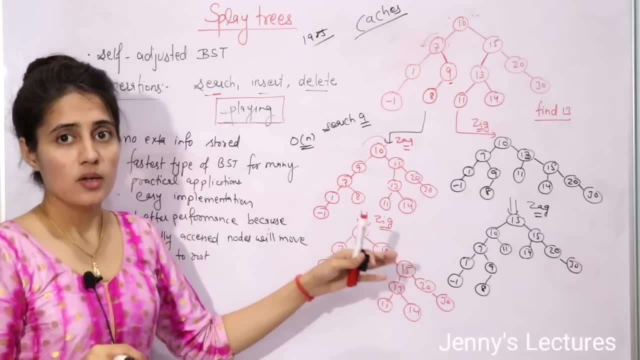 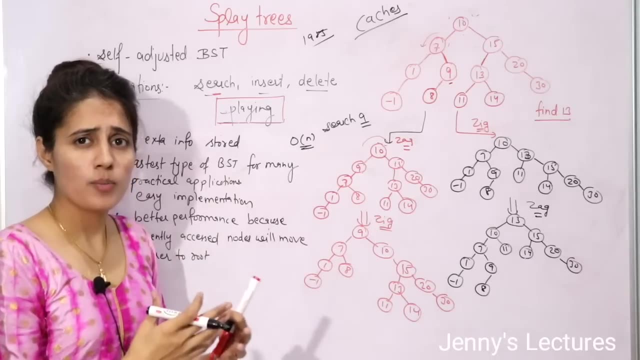 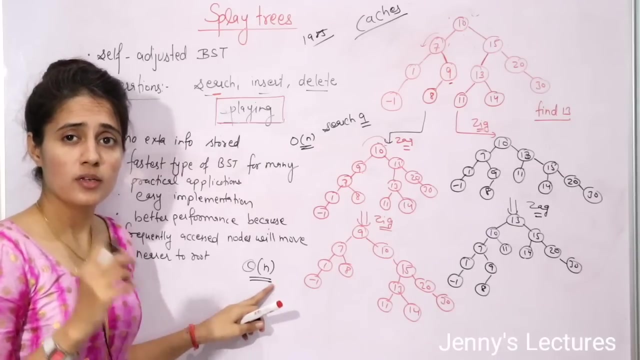 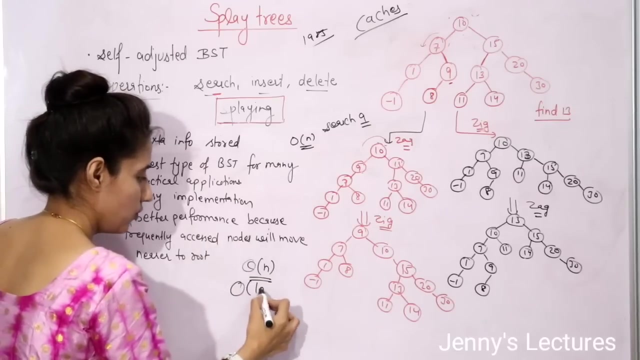 balanced trees. trees- this may be skewed, fine, but these are very. this is very rare case. so that is why sometimes any single operation may take what order of, or you can say theta n time complexity, but this is very rare case. fine, all the operations in this play tree is going to take order of. 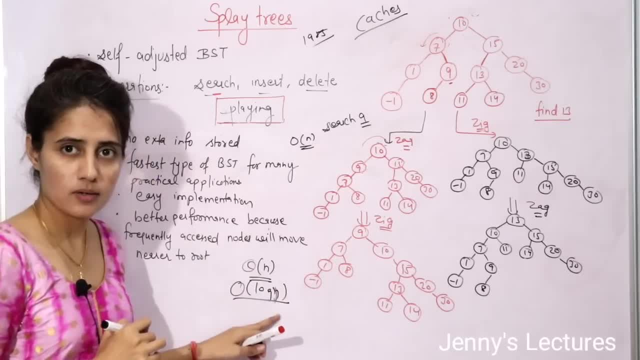 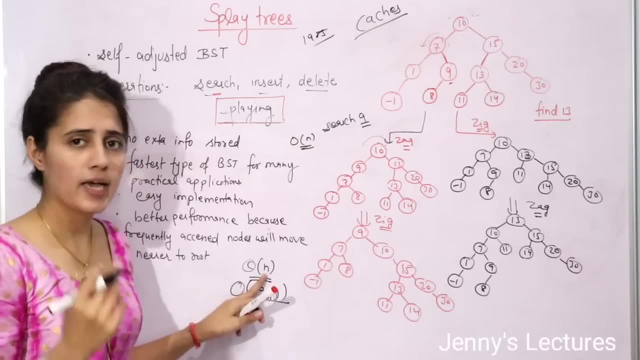 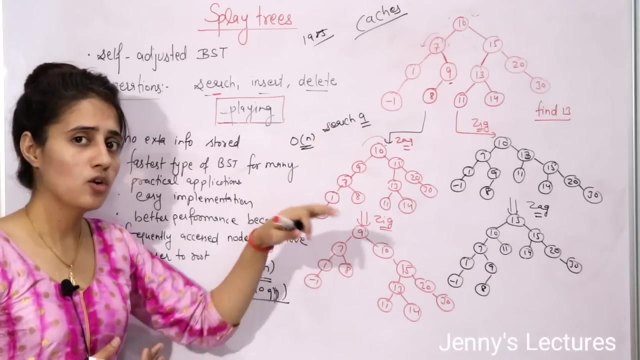 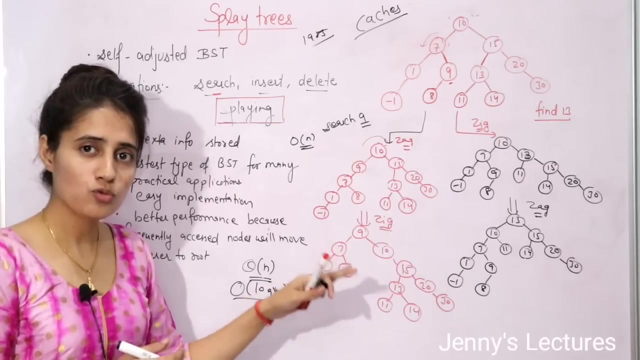 log n time complexity: right: amortize order of log n time complexity: fine: very rarely any single operation will take theta n time. complexity: fine Because sometimes the height maybe linear, I have told you because these are not strictly balanced. trees: right applications. also I have discussed that these are used to implement. 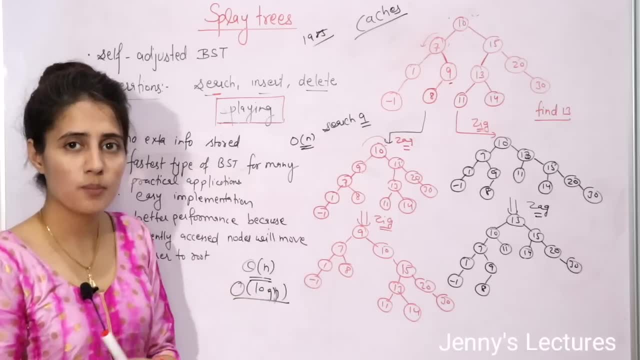 in caches, in windows and синces are used. this is a compiler Esplanade. Yes, S? nelllet Government be Douzlah, Not, for it is. So definitely those techniques, these, which, since сб, 언니 phyo Meng, Booy iye and mother team. 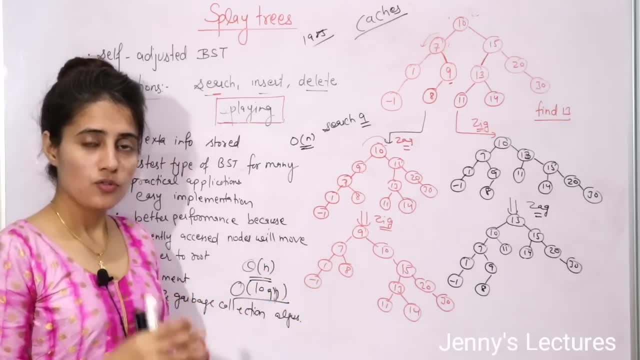 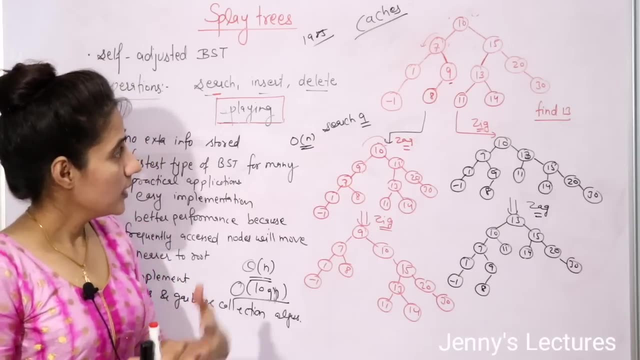 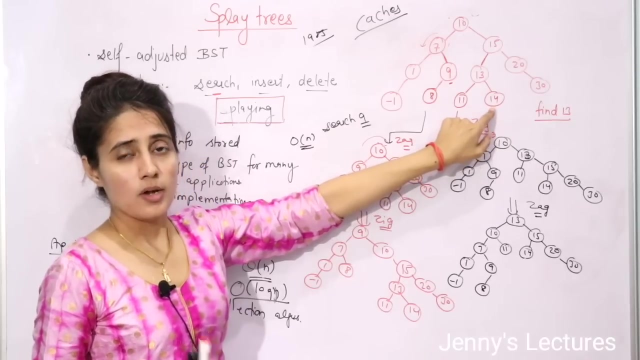 splay trees are used. so i think this is enough for introduction of splay trees. in the next video we will discuss insertion in the splay trees, right for you. the question is: suppose this is the tree. i'm taking this example and here i want to search 14. now which operations you need, which rotations? 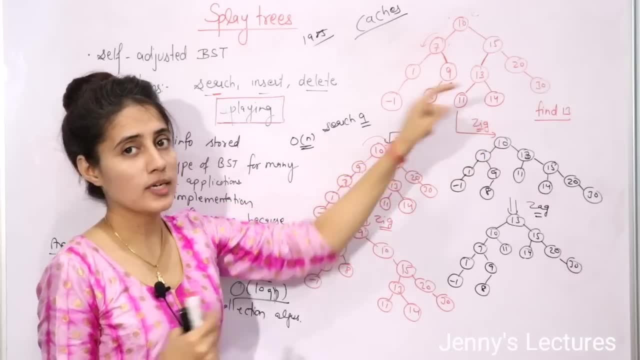 you need to require and how many rotations you require, you can tell me in the comment box. right, so now. i'll see you in the next video. till then, bye, bye, take care.